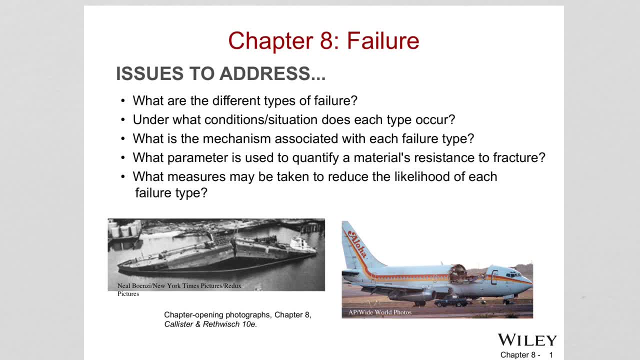 And get your toothbrush right. And this is the reason why in all packages they put a small cut for us and they say: open here. right, because when we use that region we can easily open the package. This is the underlying phenomena of fracture mechanics. So when we have a small cut, small incision or 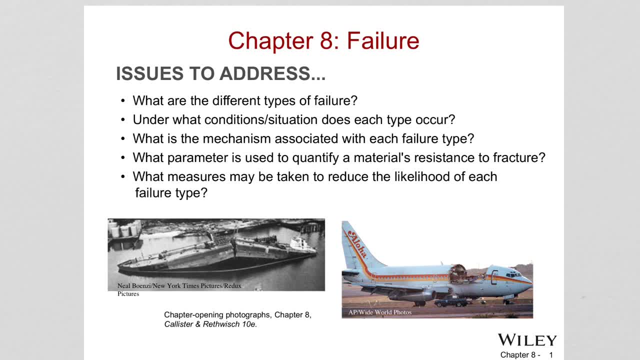 notch. This is where the stress is amplified, at the tip of this cut, and then this amplification causes the notch to propagate, to get bigger and eventually results in the failure of the material. So what we are seeing in these images? we are seeing an oil tanker, that is. 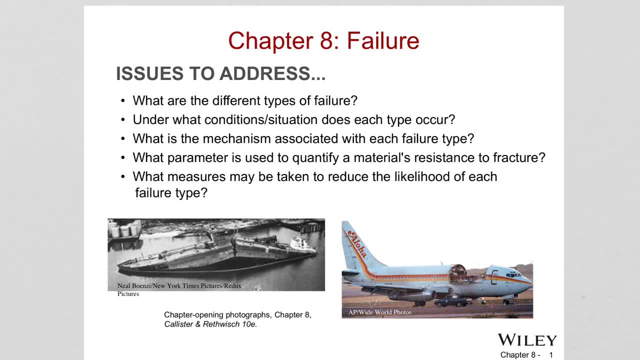 fractured in brittle manner. So brittle means suddenly. It always starts with a small notch, a small defect, small flaw in the surface, and then, without giving any warning, the material suddenly fails because that crack has propagated suddenly and we are. that's why we are seeing this damage in 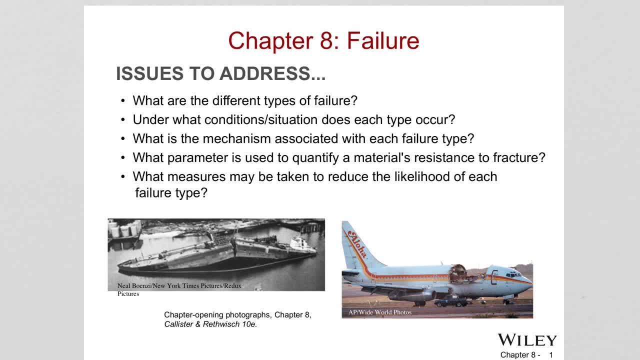 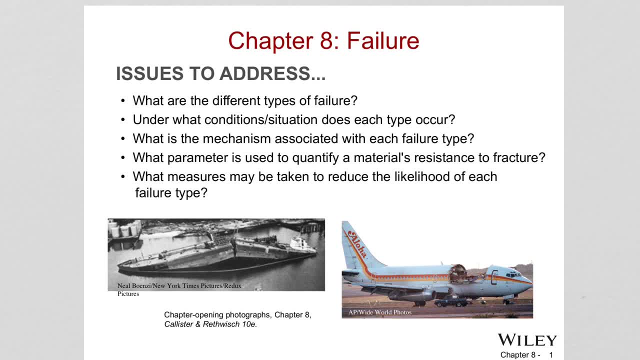 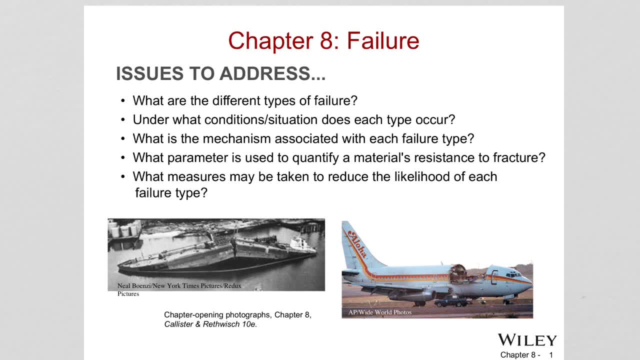 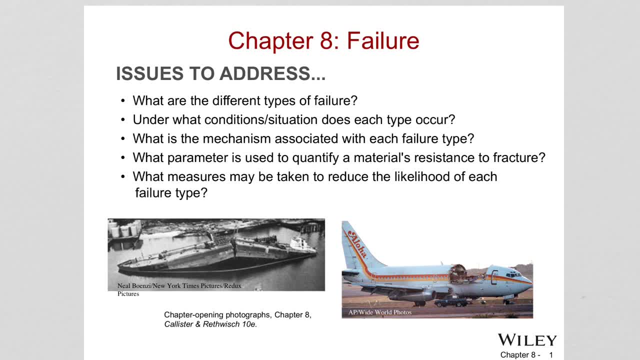 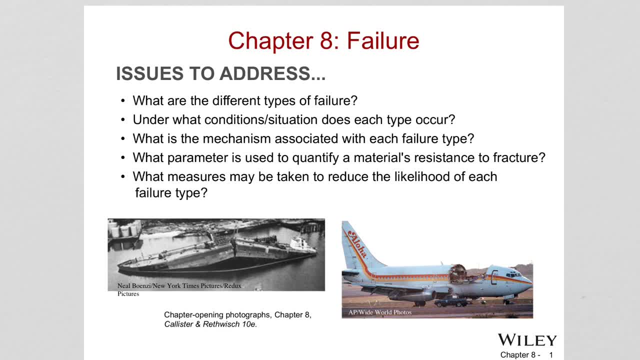 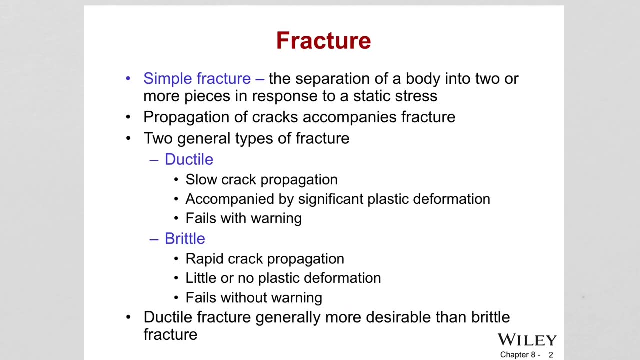 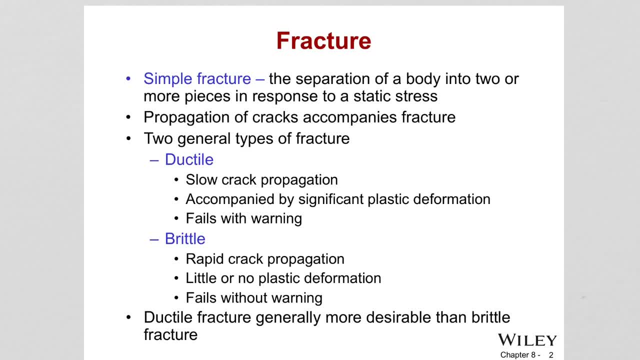 And it affects like the human lives and causes economical losses, And therefore it is an important topic to understand why materials fail and then how we can actually prevent it. So, of course, what we need to do is select materials properly, based on our knowledge of failure mechanisms and how we can prevent it. 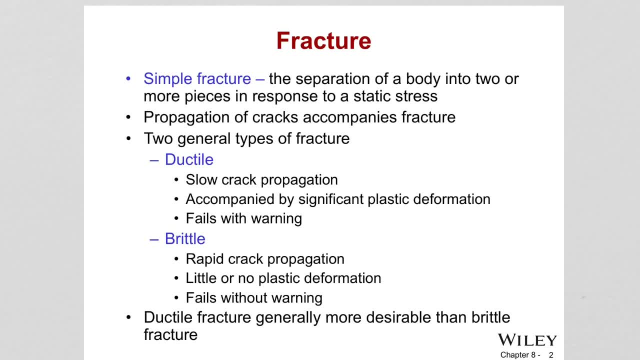 We need to choose the proper materials for that specific application. We need to be careful how we process these materials and how we inspect them. So regular inspection of the parts are also important to check for if there is any crack or any type of damage- corrosion- that is happening. 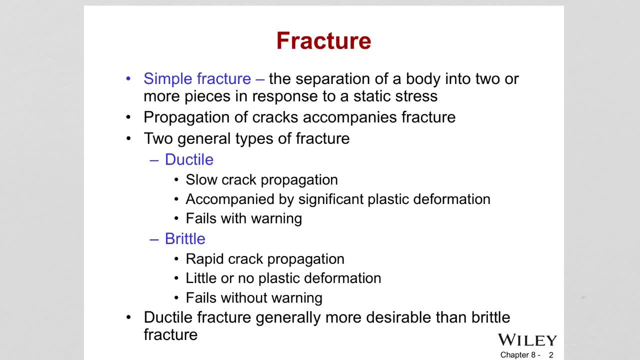 That's why usually you can, before aircrafts take off. usually they frequently actually they do some inspection, visual inspection. They use some other techniques to just to check if there is Any type of crack and because it's very important those cracks can lead to sudden failure in the material. 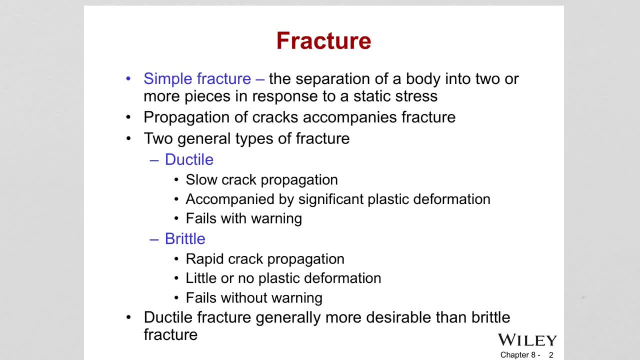 When I was doing my undergrad, my teacher once said: if you guys know how many cracks are there in an aircraft, you would never fly. So of course there will be cracks in an airplane, But we're going to later see that there is going to be some critical size of these cracks that can lead to sudden failure. 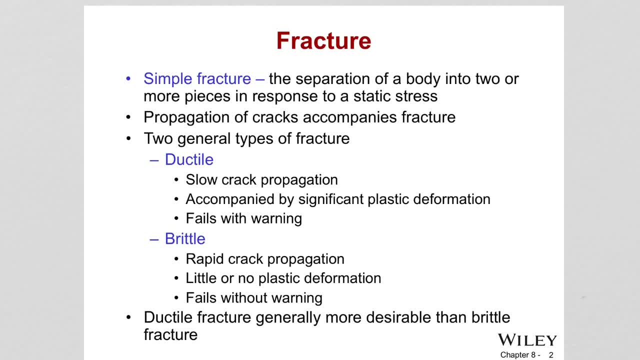 So they watch for those type of cracks. If the crack is large enough, that can lead to sudden failure. So we're going to start with basically studying the fundamentals of fracture And what is simple fracture? Fracture, it is basically separation of a body into two or more pieces in response to an imposed stress that is static. 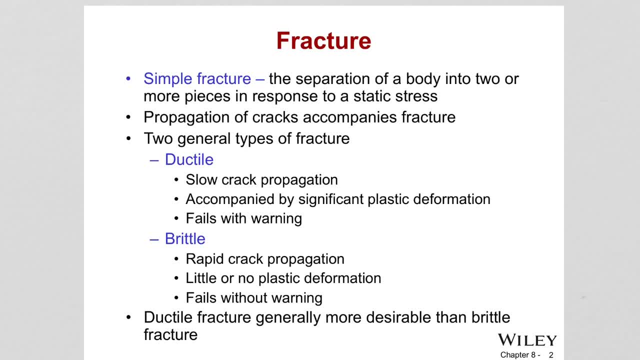 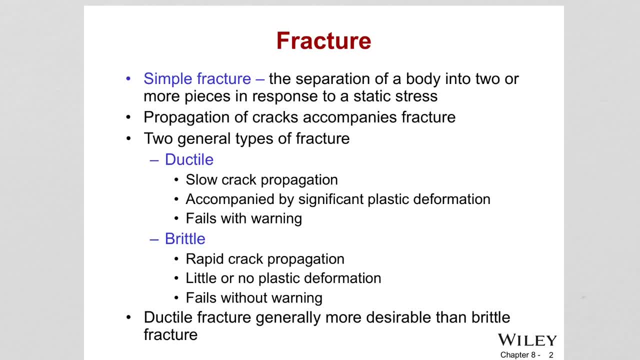 Those can happen. Creep can happen, for example, at elevated temperatures, or fatigue can happen when we expose the material to cyclic stresses. So stresses can be any type. Remember we learned chapter 6, it can be a tensile stress, compressive, shear or torsional stresses. 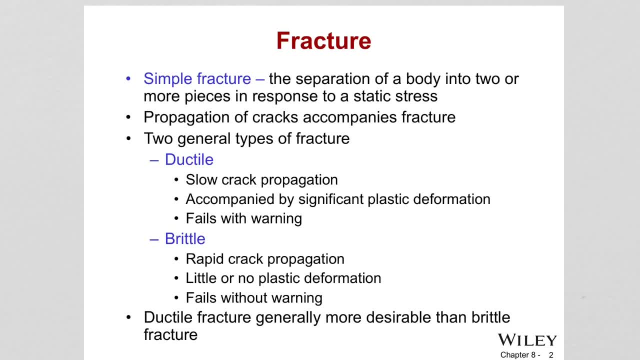 Of course any of those can lead to crack formation and propagation and failure. But in this chapter we're going to focus on usually the tensile loads and how they cause failure in the structures. For metals we have two type of fractions. 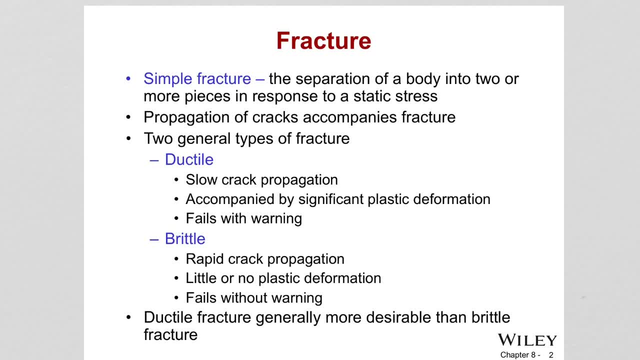 We have two fracture modes that are possible. One is ductile and then another one is brittle, So I'm sorry my dog was making strange sounds on the background. Okay, so we have ductile and brittle fracture modes. When does ductile one happen? 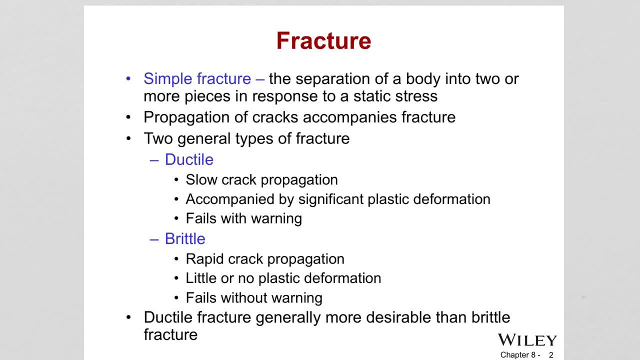 So the name implies If the metal experiences plastic deformation before it fails, then we call these ductile failure fracture. And if the material experiences very little or no plastic deformation at all, then we say this is a brittle fracture. And brittle fracture is actually the dangerous one, because it happens suddenly. 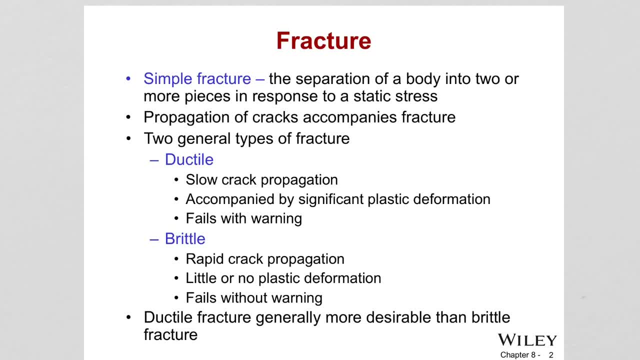 It doesn't give you any warning, But ductile one because there's a change shape, right, We can understand. it gives you some type of warning before it fails If you can visually observe the deformation region. And yeah, the ductile fracture are what we desire than the brittle ones. 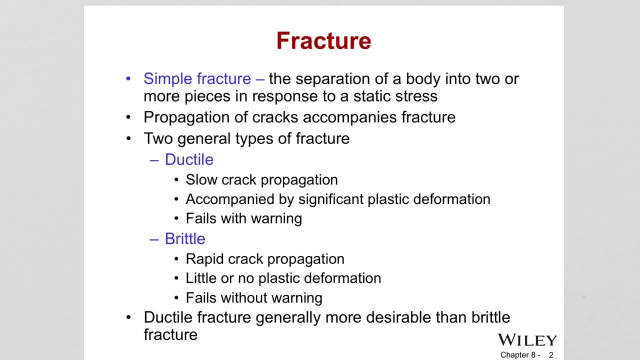 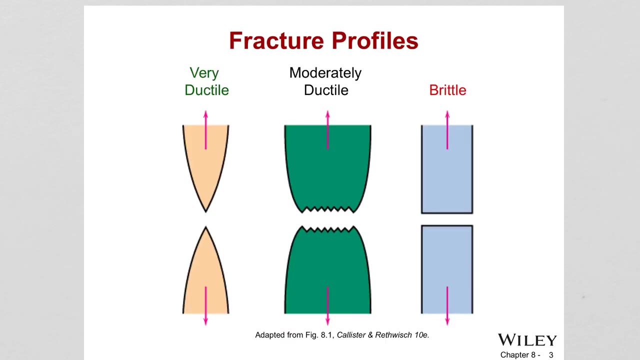 Because the brittle ones just suddenly happen And it is really bad, Like the Challenger disaster happened because of the brittle fracture of the rubber actually, or rings. So ductile and brittle fracture surfaces, they have distinctive features And both. They have distinctive features on macroscopic and microscopic levels. 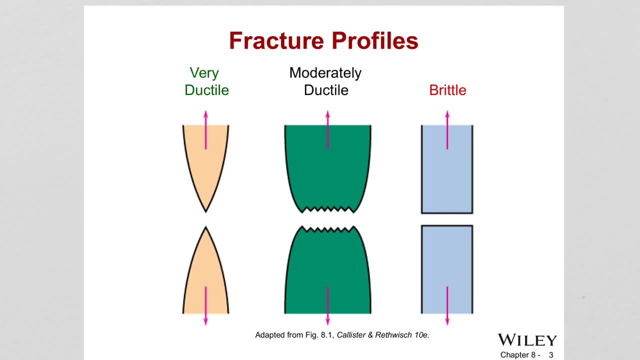 Therefore, this is how we understand if the material failed with ductile or brittle fracture, Because if we observe those distinctive features of the fracture surfaces, then we can conclude how the material behaved before it fails. So if you look at the first one, it's very clear. 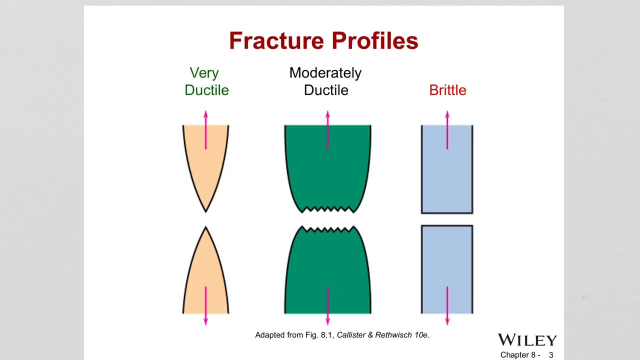 It's very clear. It's very clear. It's very ductile fracture. As you can see, there is a reduction in the cross-sectional area before the material fails. So, and there is virtually, we are seeing a hundred percent reduction in the area right. 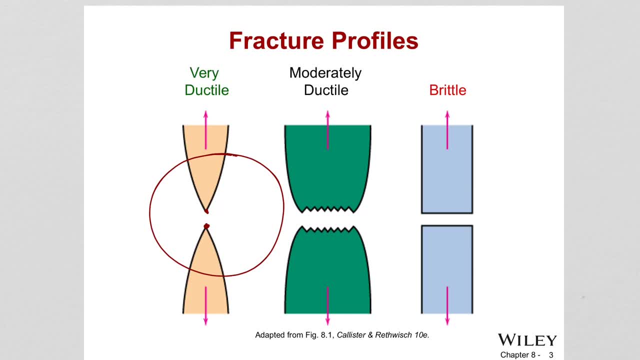 It becomes a point. So these are highly ductile material. These are very ductile, Highly ductile materials and very soft. These are, for example, gold, lead. These materials, some polymers at elevated temperature can also fail like this. 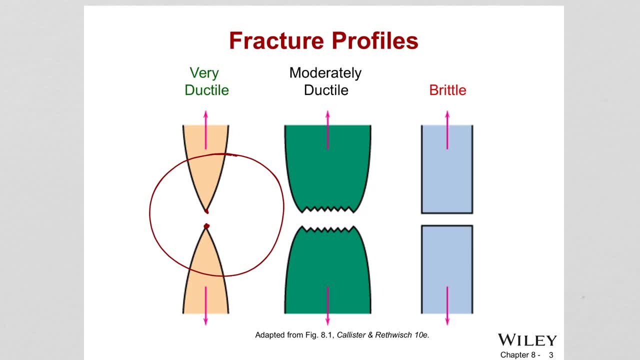 And but the most common one, the most common type of fracture happens when we have again ductile materials. It's moderately ductile materials And we are seeing this type of fracture surface Under tension. there was little moderate amount of necking, moderate amount of necking before the material actually failed. 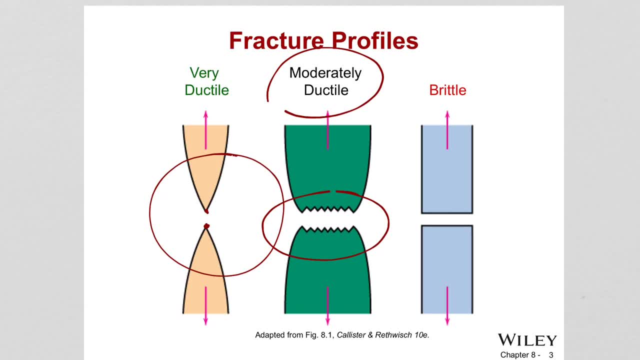 And the last one: we are seeing again ductile material. And the last one, we are seeing a fracture surface. when there is brittle fracture, As you can see, there is no necking, There is no plastic deformation, Just separation of the surfaces. basically, 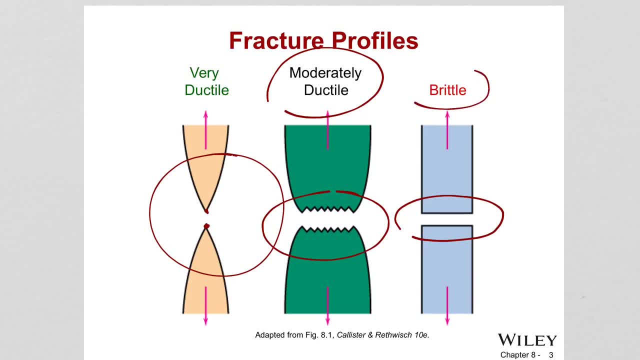 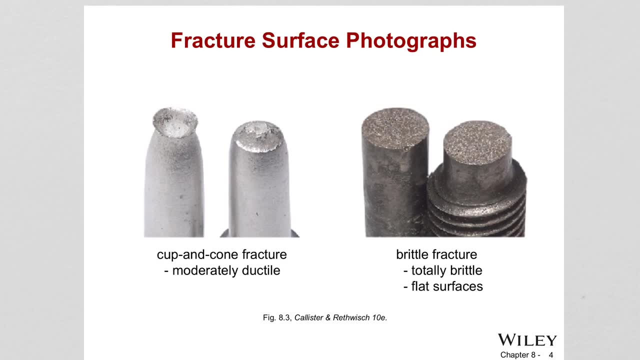 And this is how brittle fracture looks like. And this is how brittle fracture looks like. So obviously in these images of samples we are seeing a ductile fracture in the first one, because we have seen there is some reduction in the cross-sectional area and some plastic deformation happened. 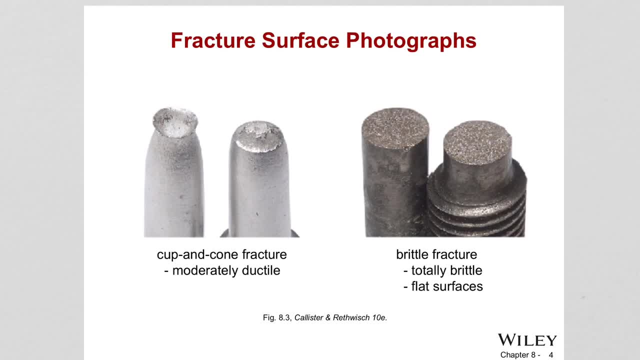 But this type of observation of the fracture surface. we can say this is a cup and cone fracture. Okay, So there is the cone and there is the cup. This is what we observed with our naked eyes And, of course, if you also do look at the surface under microscope, 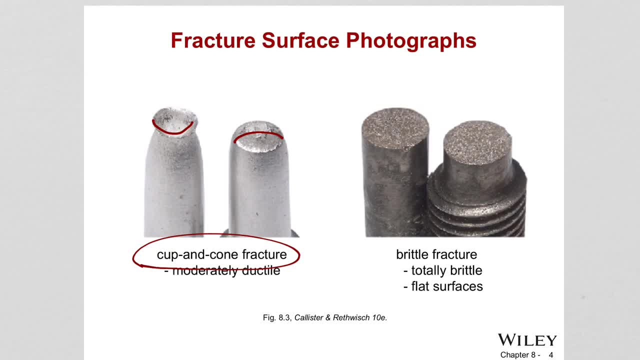 you are gonna see, the surface will have an irregular and fibrous appearance, which will be an indicative of a plastic deformation. On the other image we are seeing an obviously a brittle fracture. So you can see there is no plastic deformation at all and the surfaces are flat. 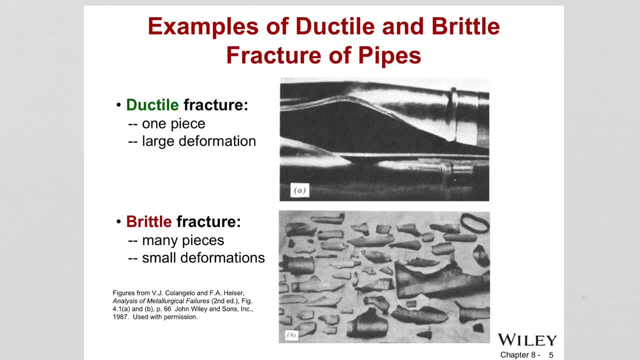 Another difference between ductile and brittle fracture is: think about when you have glass or ceramic cup. those are brittle materials, right. when you drop them, or when you drop them on the surface, they are flat and they are not. When they shatter, they are broken into many pieces. 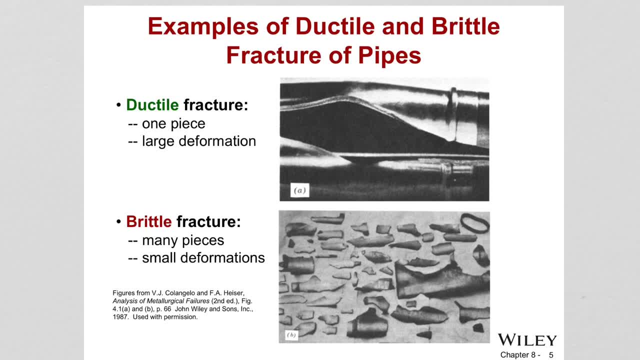 That is brittle fracture, Whereas the ductile fracture, the material preserves its wholeness. So we see one piece, But it's a large deformation. But in brittle fracture that is small deformation. so many deformations, Many pieces, but small deformations. 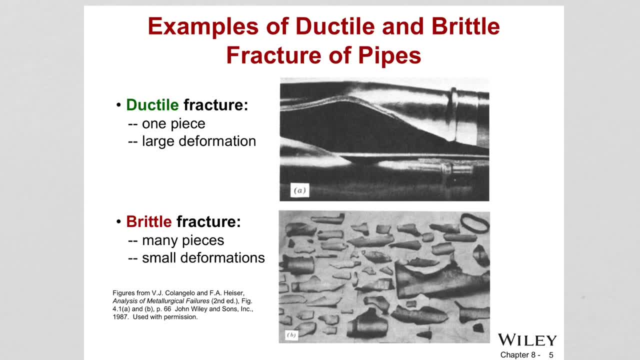 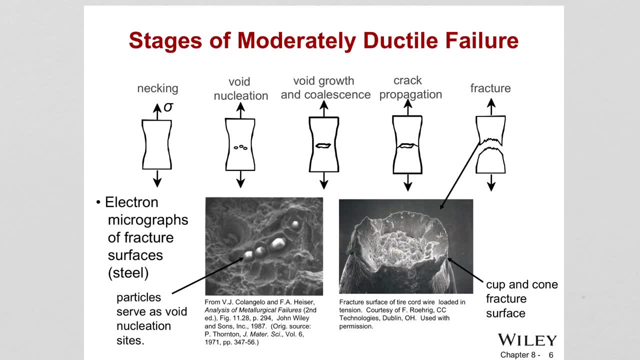 That's what we see. So there are steps to the failure, And it always starts with the crack formation first, And then this crack then propagates, causing the fracture. So we see the fracture, So we see the fracture. So we are seeing here the stages of moderately ductile failure. 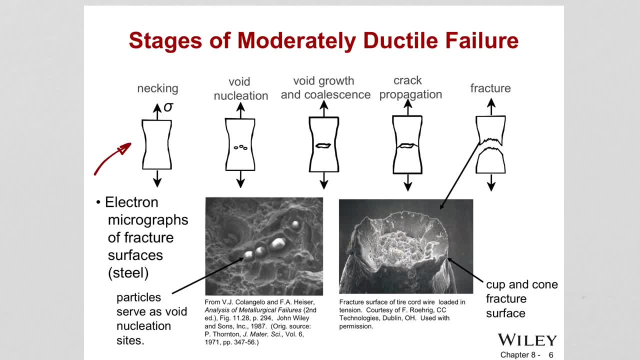 And first, under tension, necking starts And this necking will be the reason there will be small cavities or micro voids will form in the interior regions of the cross section, Like we are seeing here. There are reasons why voids can happen. 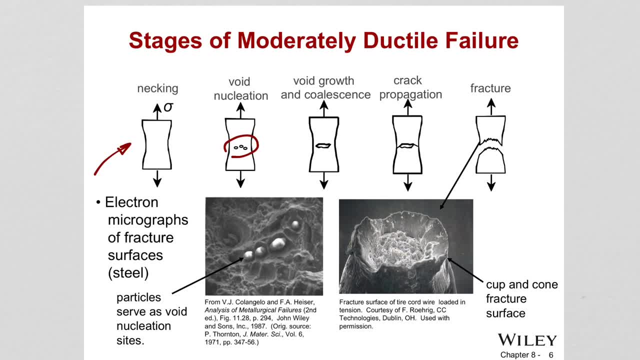 Those can be defects like inclusions. Inclusions means some oxides in the structure that are trapped. Those type of defects can be the reasons why actually voids can nucleate and form in the necking region. So after this, as we continue to deform the material, 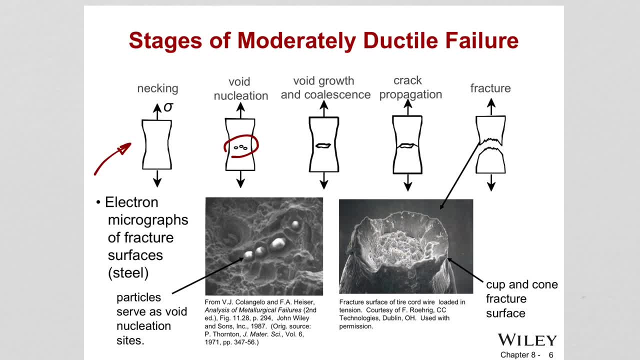 the voids will. The voids will enlarge and they come together, they coalesce to form an elliptical crack, like we are seeing here. And these are of course, as you might notice, perpendicular to the stress direction, Because the crack formation is happening like this, but the stress is applied perpendicular to that. 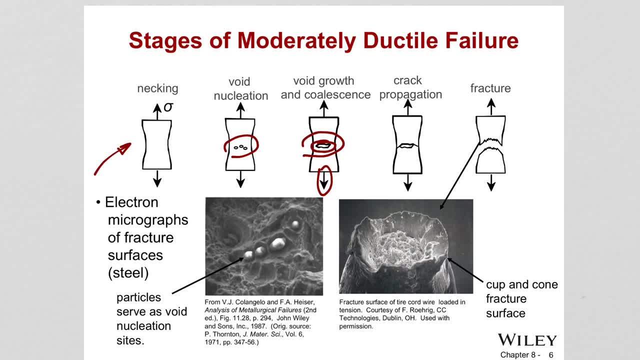 And once this crack exists in the structure, what is going to happen? by the application of the stress crack will continue to grow and propagate along the cross section. And finally, of course, we observe the fracture. And of course, finally, fracture happens due to the propagation of the crack. 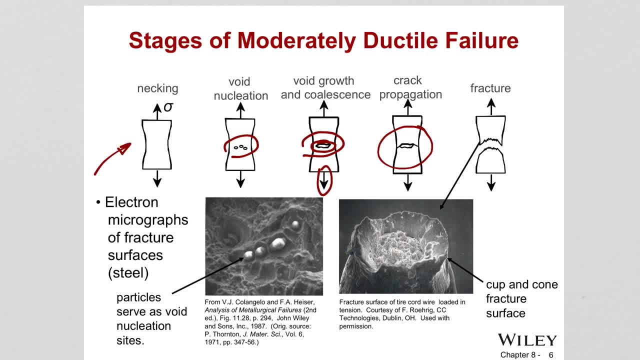 But we noticed the propagation of the crack around the outer diameter of the neck happens by shear deformation at an angle about 45 degrees. So remember 45 degree is when the shear stresses are maximum. This type of fracture is resulting in a surface morphology, what we call cup and cone fracture. 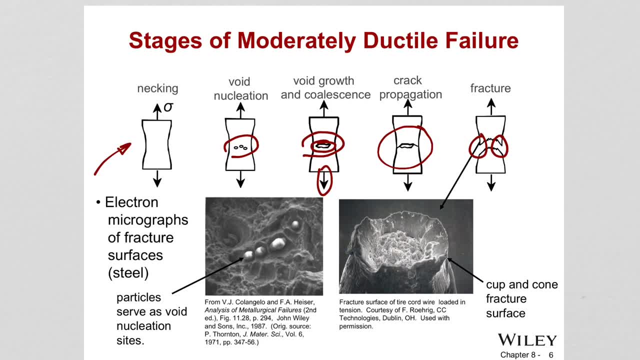 So when they analyze under microscope how these fracture surfaces looks like, they can see the particles that were the reasons why voids form in the first place. I told you, guys, these can be some impurities, the fact that are introduced during the production of the material, or it can be coming from the raw material. 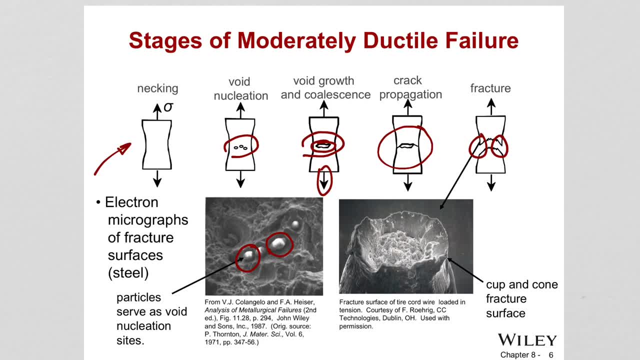 Some oxides, Some hard particulates. These are the reasons the voids form in the first place, under tension, Of course. once a void forms, it propagates by continuing application of the tension And therefore, once it propagates, the failure happens. And we are seeing under microscope how this cup and cone fracture surface looks like. 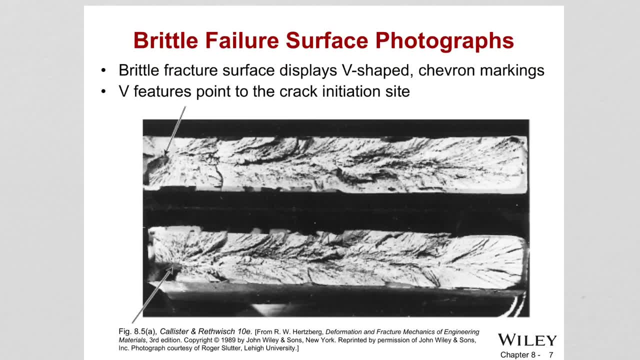 So how about bridal failure surface? How does it look like? First, we learned that there is nearly no plastic deformation observed And the surfaces are flat. And in some steel pieces, v-shaped Charon markings may form at the origin of the fracture. 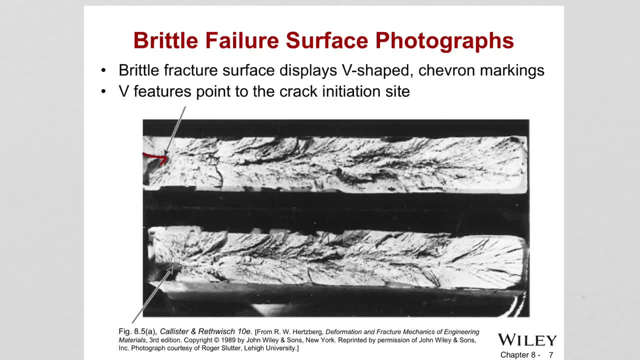 The origin of the crack, Like we've seen, And in some cases we see lines that radiate from this origin of the crack, Like this, And these are indicative, Indicative, Indicative of the bridal fracture, basically, And these can be visually seen with the naked eye. 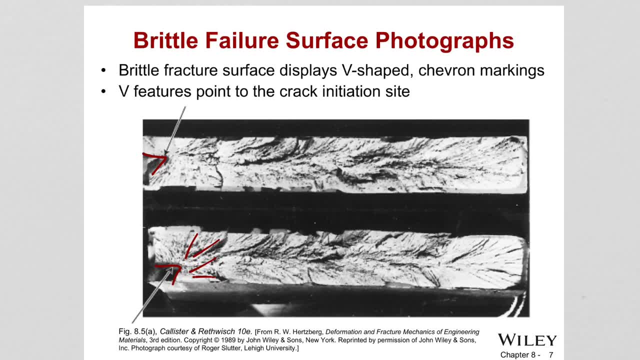 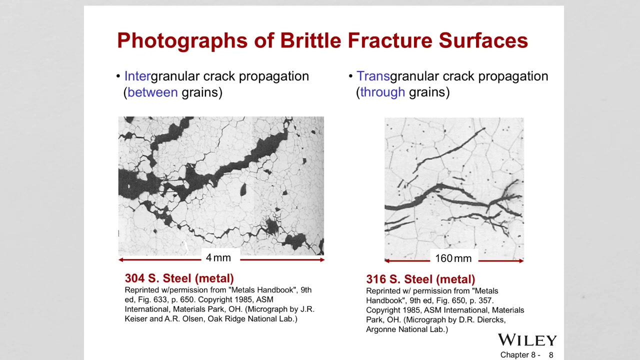 In some materials there might not be any discernible fracture pattern And when it is, in the case of amorphous materials, They are bridal fracture. Ceramics, glasses: They yield a relatively shiny and smooth surface. So those observation tells us The failure happened with bridal fracture. 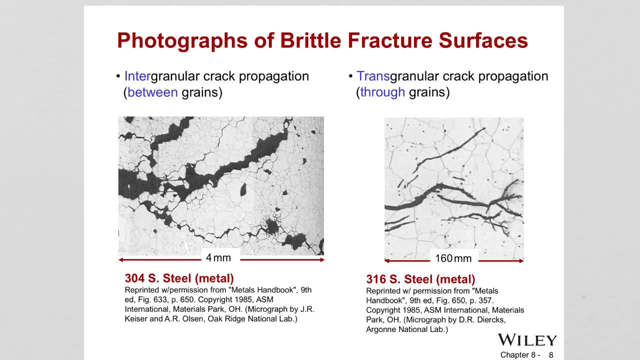 So for most bridal materials, Crack basically propagates. Remember the first: it has to form, There has to be a crack, And then it propagates By the breaking of atomic bonds. So this process is called cleavage And when this happened by just the breaking of the atomic bonds. 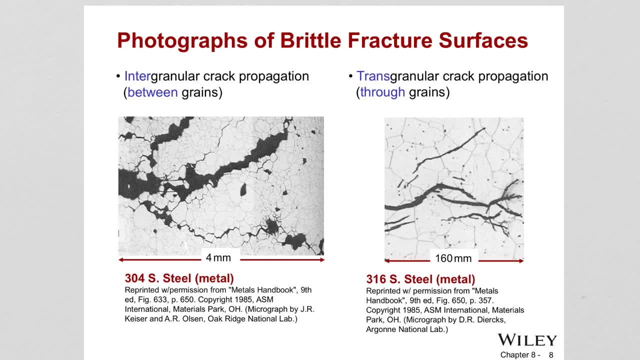 Then this fracture is said to be transcrystalline or transgranular crack propagation, Which happens through the grains And here under microscope. When they observe how the grain structure looks like after the failure, You can see the grains Right. 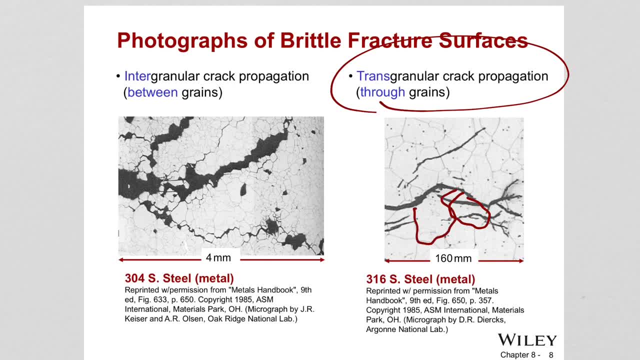 These are individual grains And the crack has gone through. You can see here. The crack has gone through Individual grains, Through the grains. That's when we call transgranular crack propagation. In some alloys, In some metal alloys, We observe 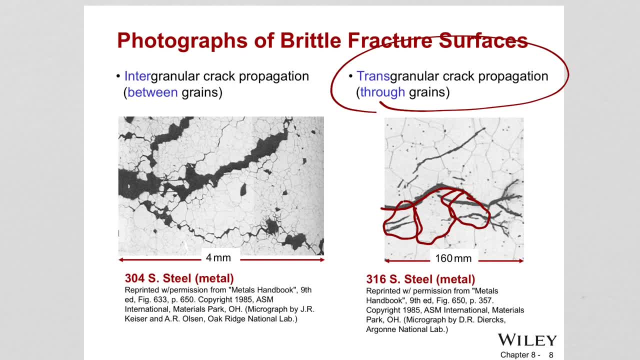 That crack actually propagated along the grain boundaries. Like we are seeing here, It's not going through the grains But it is happening in between the grains. So the crack propagation happening Along the grain boundaries, This is what we call Transgranular crack propagation. 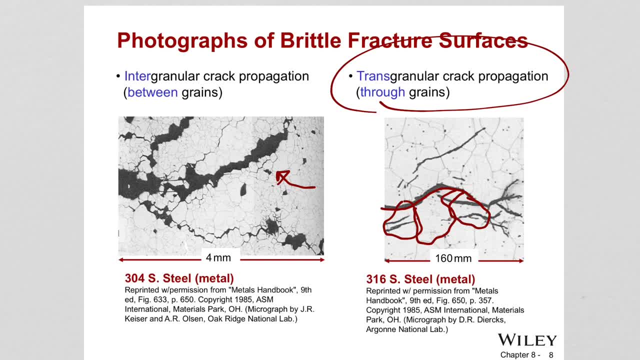 This type of behavior observed If there was any process that has weakened Or make the grain boundaries brittle. That's when we observe Such crack Morphology Um. 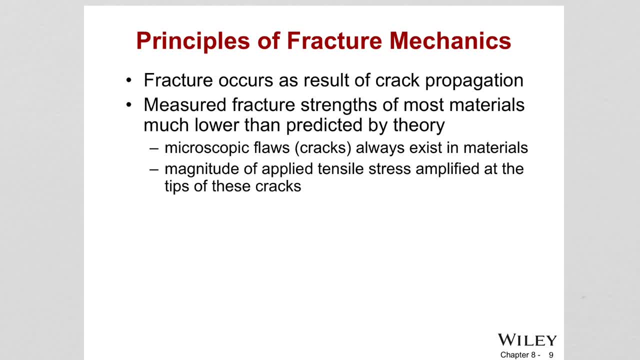 Now we are going to take a look at Principles of fracture mechanics. So fracture mechanics Is a field That research Basically The failure of materials And gives us relationships Between material properties, Stress level, The presence Of Flows. 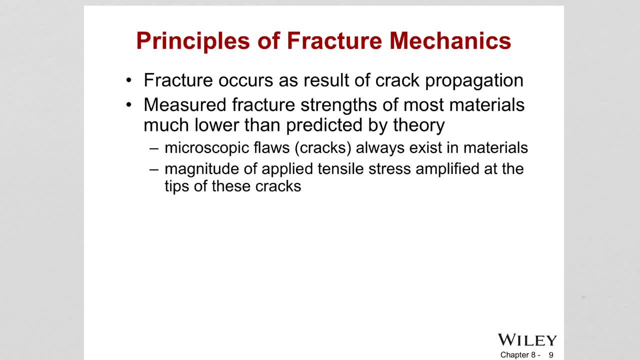 That can propagate And their propagation mechanisms. So Again, Fracture occurs As a result of crack propagation. So first there has to be a crack And then Failure happens When the crack propagates. Okay, So When they measure, 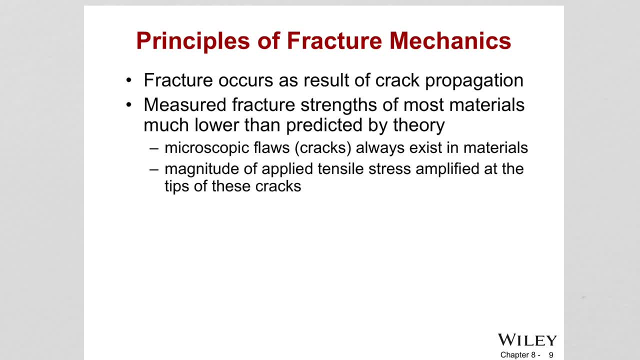 The fracture strength Of most metals. Theoretically, We have seen that In actual life, Those fracture strengths Are actually much lower Than what we can predict With equations, And this is due to the fact That there is 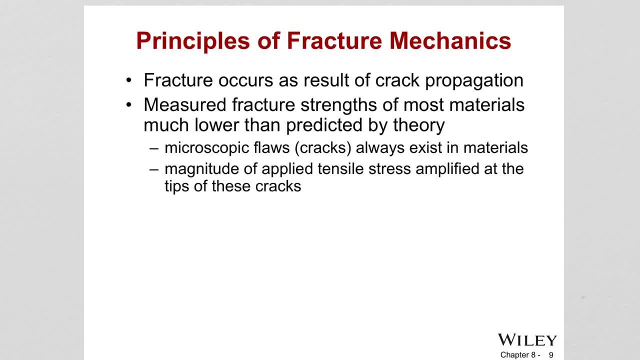 Always Cracks Exist In materials. There is never a perfect Material And these Cracks Always Exist In materials. There is never a perfect Material And these Cracks Always Exist In materials. 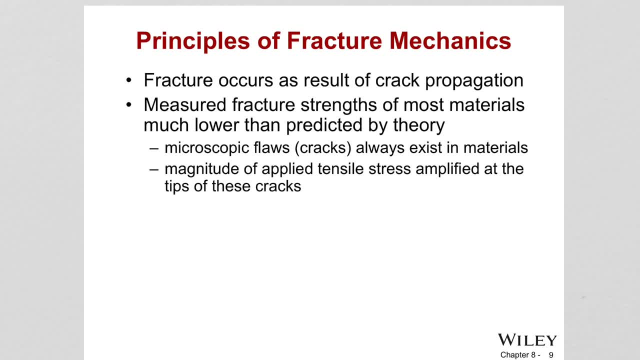 And these Cracks Can be Introduced During the Manufacturing Of that Material, And Also The Magnitude Of the Applied Tensile Stresses At the Tip Of these Cracks. 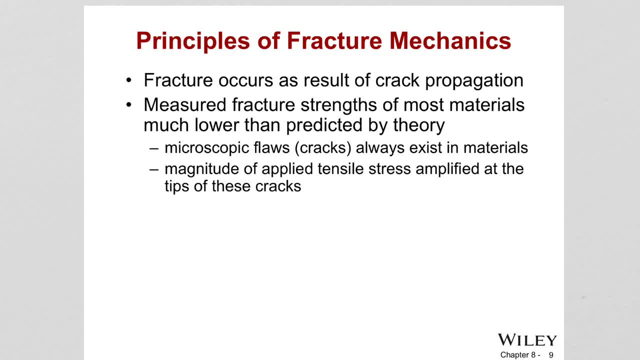 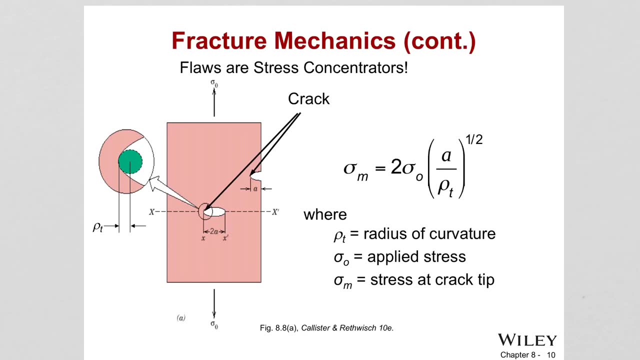 Will Be Much Higher Than What We Are Going To Understand That Concept. So When There Is A Flaw Or Some Crack In The Material, 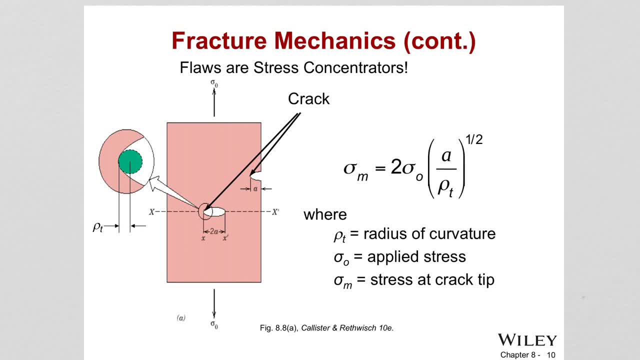 It Can Be Inside, Like We Are Seeing Here, Or It Can Be Any Way, When There Is Cracks Like These Present In The Structure. 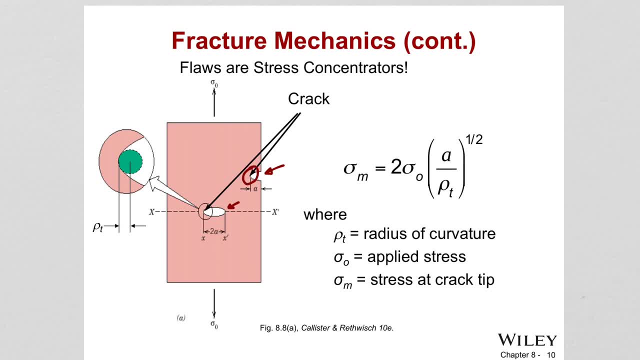 They Will Act As Stress Concentrators, So It Will Be Much Higher The Stresses Around That Crack, Near The Crack, And How Much It. 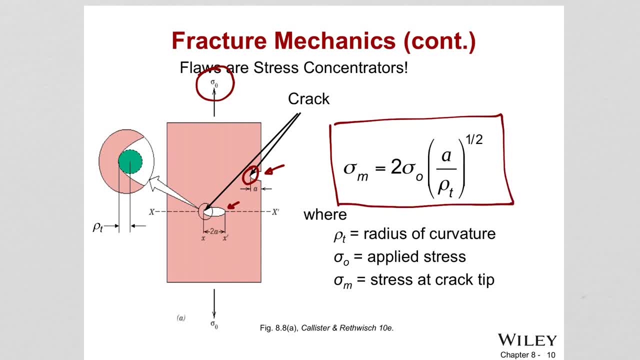 Is Amplified Near. The Crack Is Given To Us With This Equation, Because It Is Important To Understand The Stresses Next To Understand So Here. 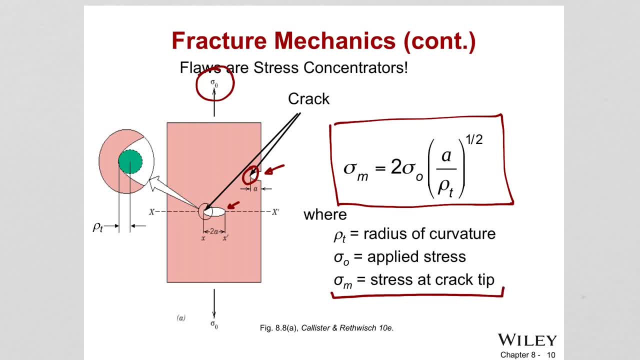 Sigma M Is The Stress At The Crack Tip Okay And Sigma Not. Is What We Actually Apply To The Material And Roll With The Subscript. 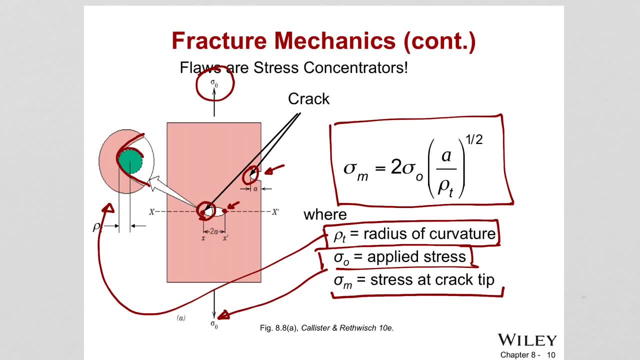 T And Assuming It's Close To A Circle, We Are Getting The Radius, Radius Of That Curvature Okay, And You Are Seeing That, The Dimensions. 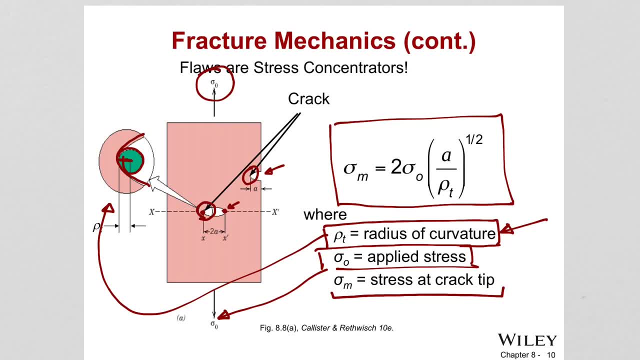 The Geometric Configuration Of The Crack. So Much Of These Applied Tensile Stress Is Amplified- Depends On The Crack Size, If It Is A. 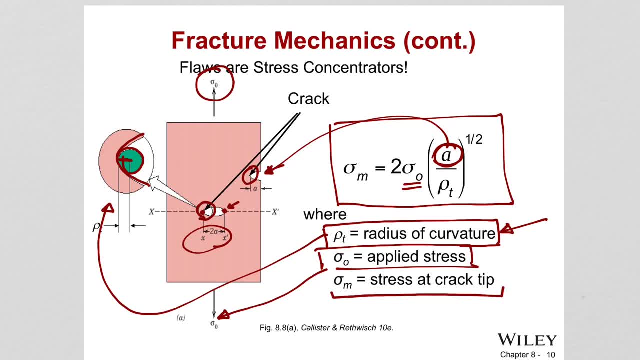 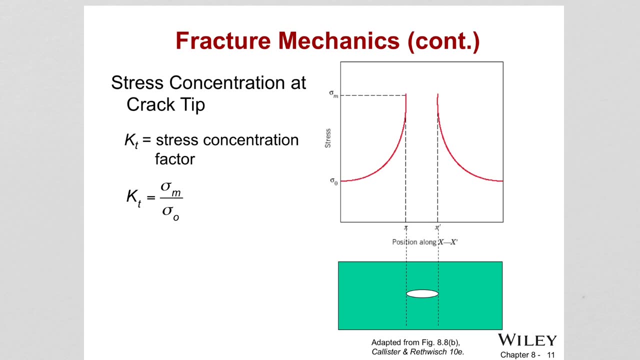 If It's Outer, Even If It's To A Inner Crack, You Are Here In The Equation. So All Those Relationships Are Found Basically By Experiments. 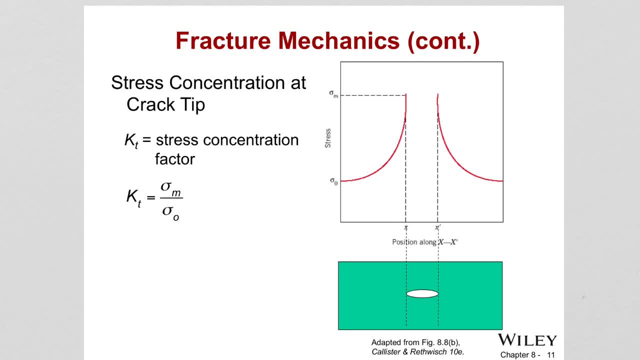 They Found Those Relationships Between The Curvature Of The Crack Tip And Therefore, What Is The Stress Arises Next To The Crack Tip, So Next, 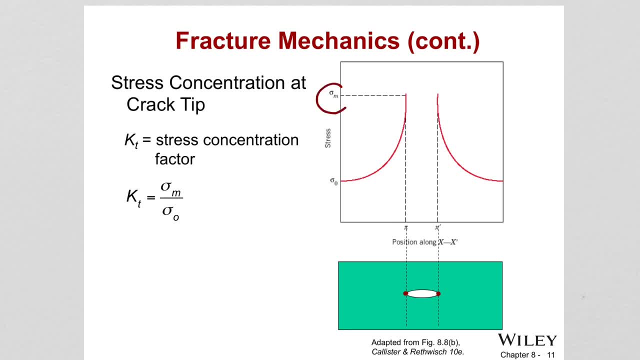 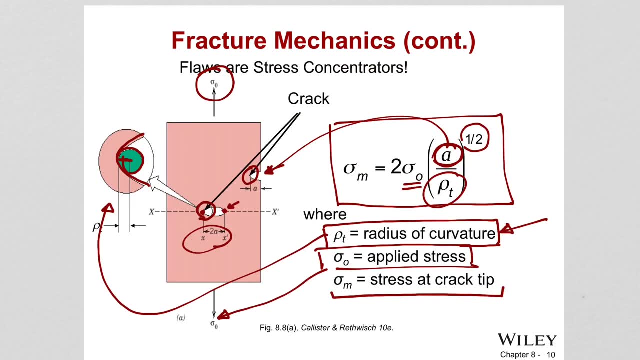 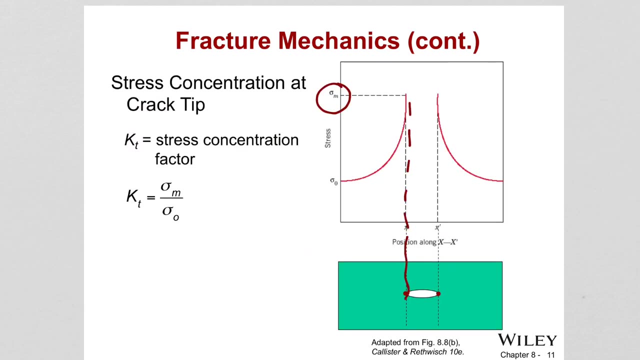 To The Crack Tip, We Reach A Maximum Stress. So This Is Called The Stress And Next The Crack Tips. They Are Reaching A Volume. 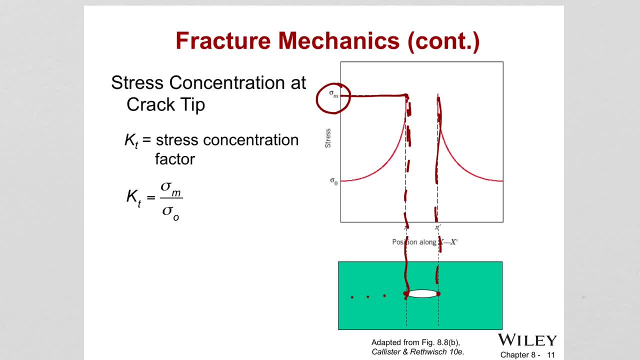 Of Sigma M And As We Move Away, As We Move Away From The Crack Tip, Stress Is Decreasing And Coming To The Crack Tip. 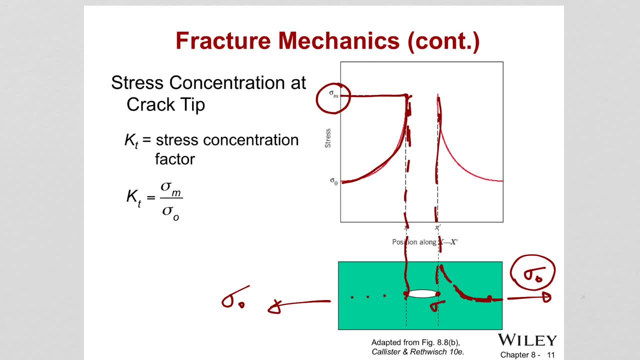 Here The Material. This Point Experiences Sigma M, So Therefore We Can Define How Much It Is Amplified Right. The Stress Concentration Factor: How? 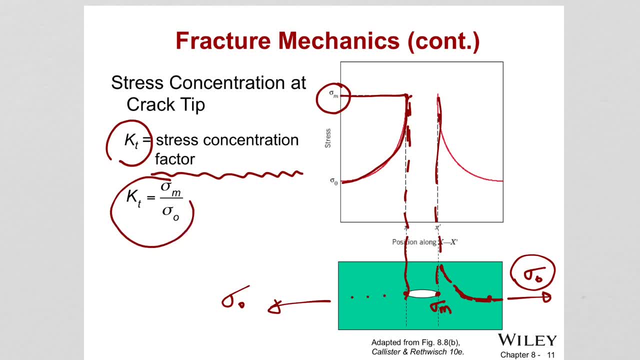 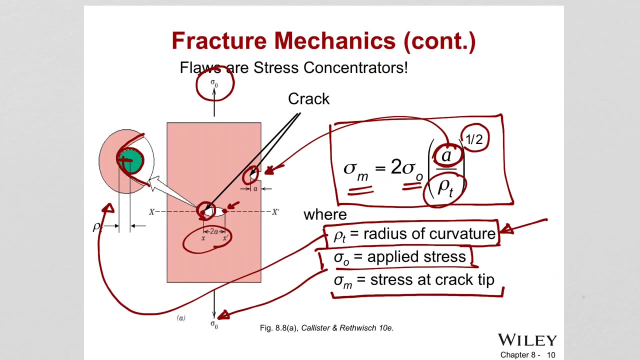 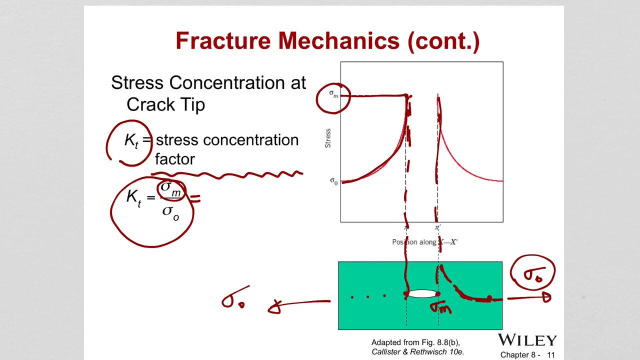 Much We Do Is Equal To Sigma M, The Stress Next To The Tip Over Sigma Not, Which Is The Applied Stress. And Since We Know 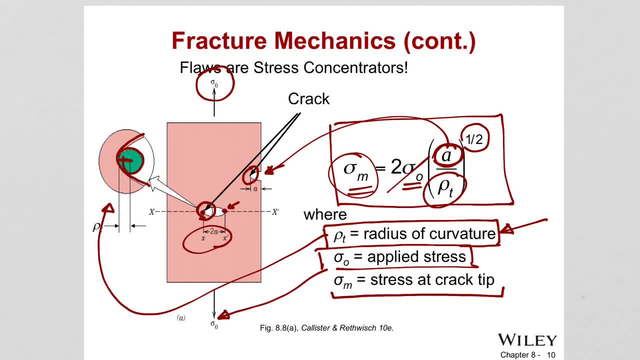 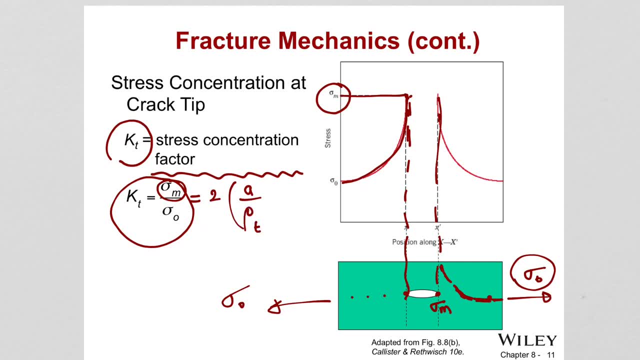 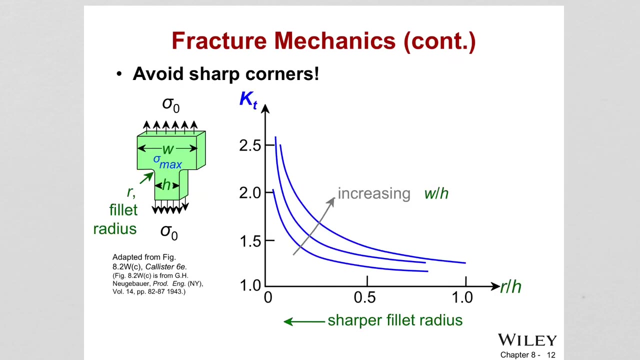 The Equation With: For Sigma M Is Two Times A Over Rho, To The Power Of One Over Two. So This Is What We Call. 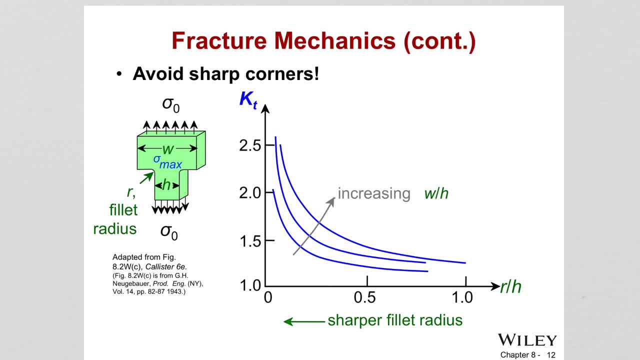 Stress Concentration Factor. So Geometric Discontinuities Cause An Object To Experience In Stress, Like Sharp Internal Corners Holes, Sudden Changes In The 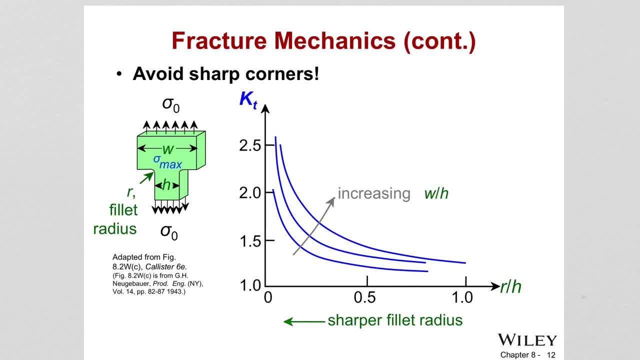 Cross Sectional Area Scratches Cracks, And That's Why, Usually, We Are Told To Avoid Sharp Corners In The Structures And In The Chart. 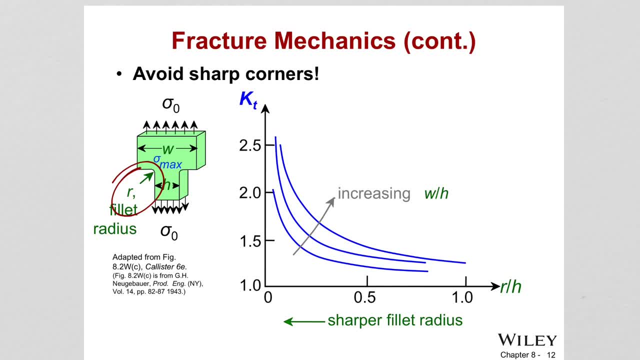 We Are Also Seeing How This Stress Intensity Factor, Or Stress Concentration Factor, Actually Increases As We Go To Sharper Fillet Radius, Because R 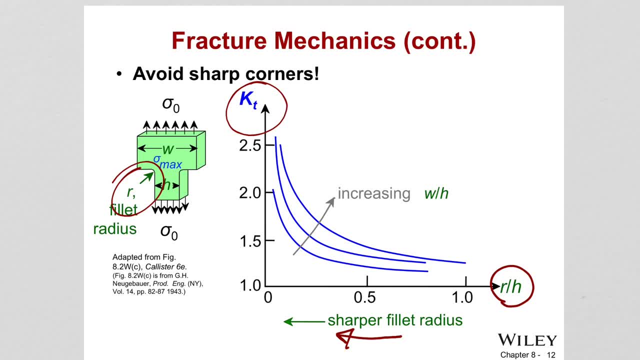 Is Decreasing. We Have Sharper Corners And This Increases The Stress Concentration Factor, Meaning You Are Amplifying The Applied Stress To Larger Volumes. 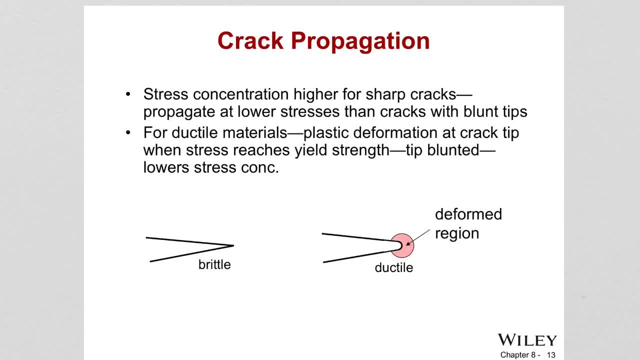 Near Those Corners. So Let's Now Look At Crack Propagation. So We Have Just Learned That We Have, If We Have Sharp Cracks, That 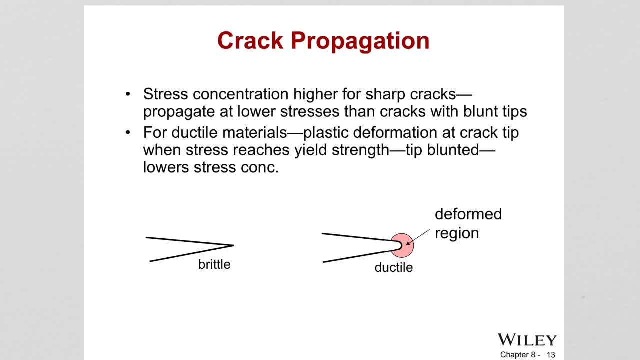 Will Increase The Stress Concentration Factor. Therefore, If Stresses Low Stress Volumes, It Will Be Amplified To A Volume That Will Cause The Crack. 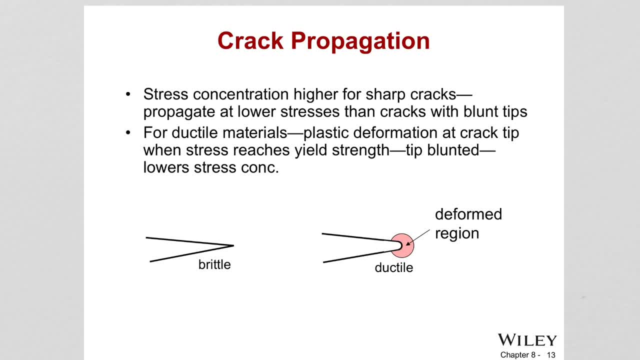 To Propagate When Compared To Blunt Tips, Where Less Stress Concentration Factor Will Be Increased At The Crack Tip. Because What Happens Here Is: 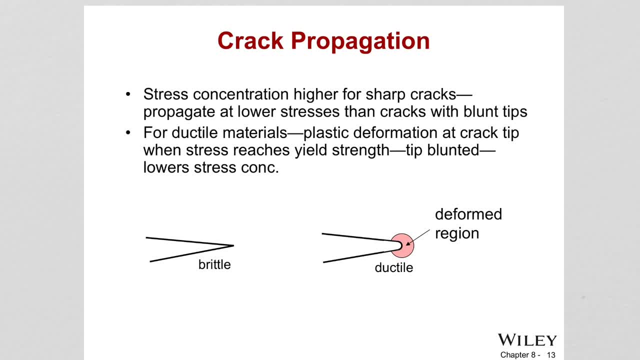 Remember, We Are Reaching The Yield Strength Of The Material First For The Plastic Deformation To Take Place, So At, Therefore, What's Going To? 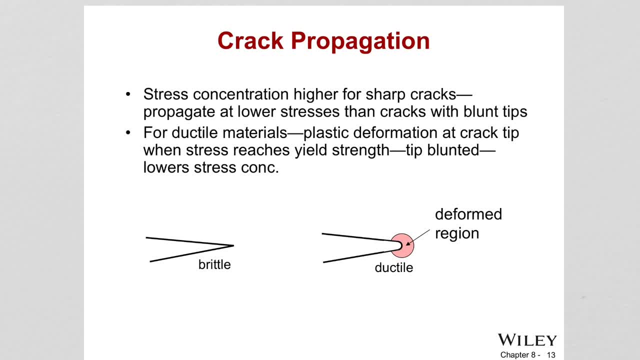 Happen In The Vicinity Of This Crack Tip, There Will Be Plastic Deformation Taking Place. So We Have Learned Two Things Here: Sharp Cracks. 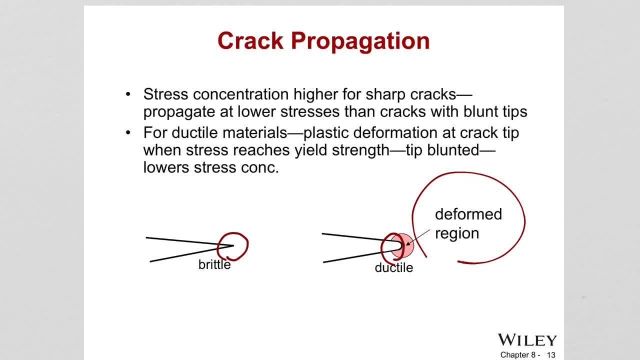 Compared To Magnitudes And When There Is Ductile Crack, Ductile Material, That Will Experience Plastic Deformation At The Crack Tip. But In Brittle 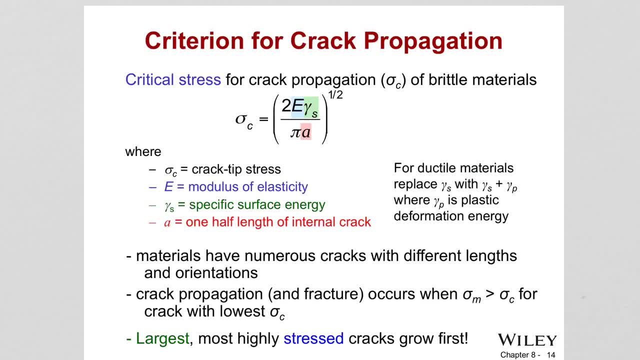 Material. There Won't Be Any Plastic Deformation. What Is The Stress Required For The Crack To Propagate? We Call This The Critical Stress, Which. 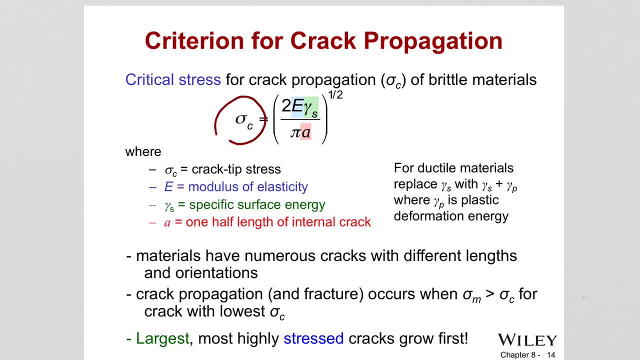 Is Causing Crack To Propagate In A Brittle Material. So That Is Causing The Crack To Propagate Basically, And There Is Also E. 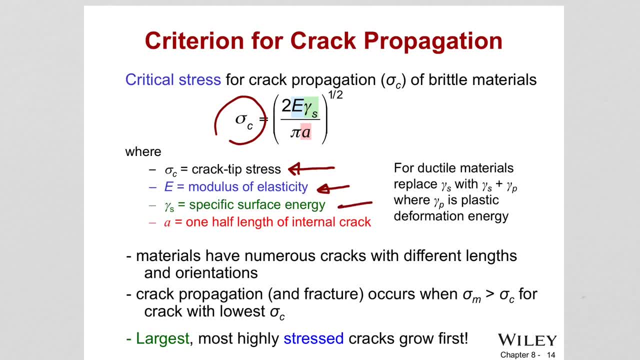 In The Equation, Which Was The Modulus Of Elasticity. And There Is Surface Energy And There Is One Stress, Which Is The Stress That Causing 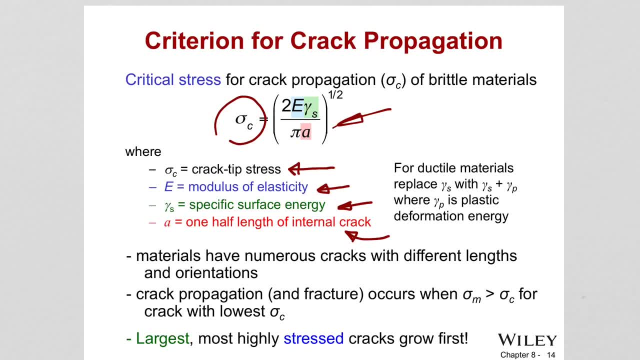 Crack To Propagate In Brittle Materials Depend On First The Modulus Of Elasticity, Which Will Change Depending On The Material And The Thermodynamics. 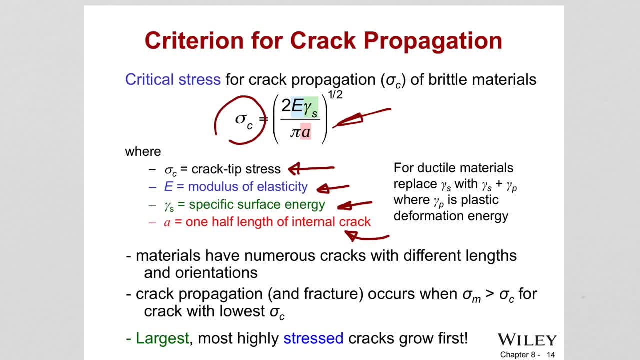 Of Energetics, Of Crack Propagations When These Cracks Become Stable Enough To Propagate. Basically Because Each Time You, If Each Time The 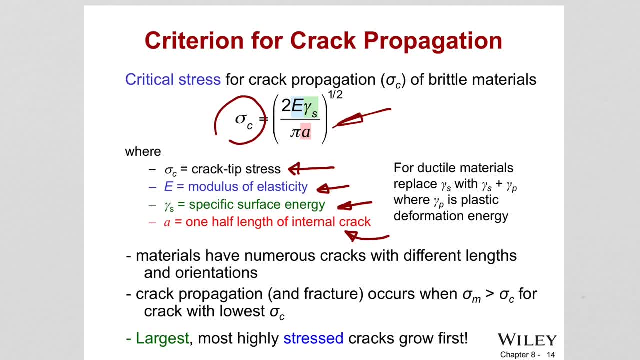 Crack Propagates One Step. Remember There Is When You Are Generating The Surfaces, And To Generate Those Surfaces It Requires To Provide Some Surface. 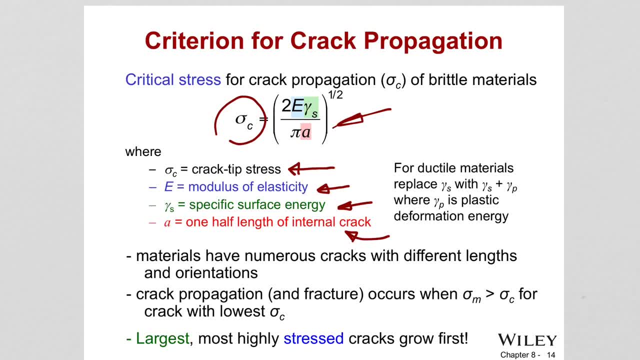 Energy. So For Brittle Materials There Is Just Surface Energy Term Comes From Plastic Deformation Next To The Crack You Also Need To Add Plastic. 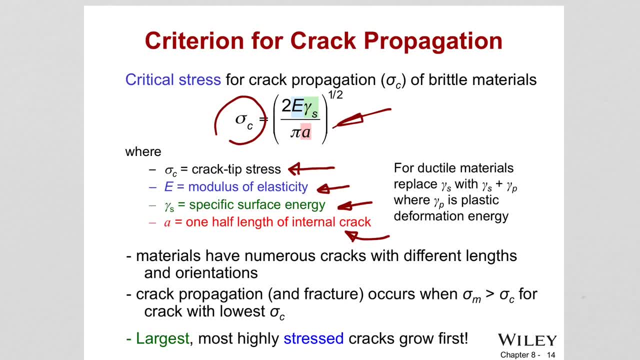 Deformation Energy, Because As We Deformed The Material Plastically, We Are Also Storing Energy. Right, We Have Plastic Deformation, There Is Also Energy. 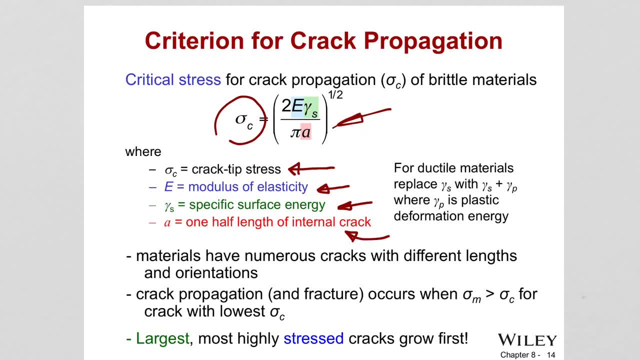 Is Related To That Plastic Deformation, So Materials Will Have A Lot Of Cracks And All Of These Will Have Different Lengths In Brittle. 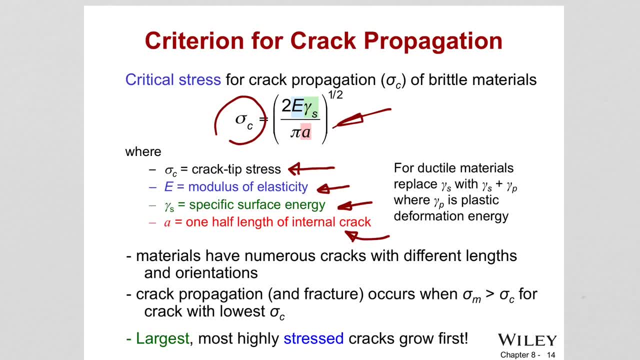 Materials, Then It Will Result In A Fracture. Okay, So Crack Propagation And Therefore Fracture Occurs. When You Go Above That Critical Stress. 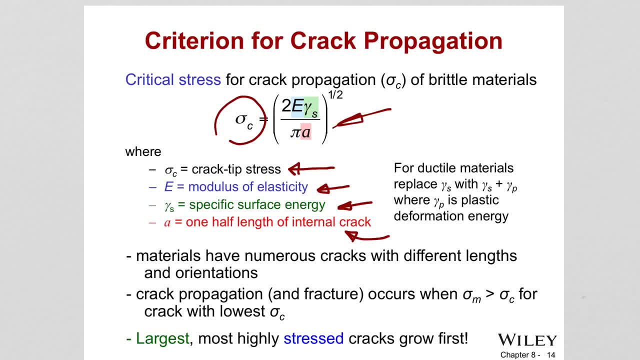 Next To The Tip Of The Structure, It Will Only Happen To As One Of Those Cracks Where It Requires The Lowest Amount Of Critical. 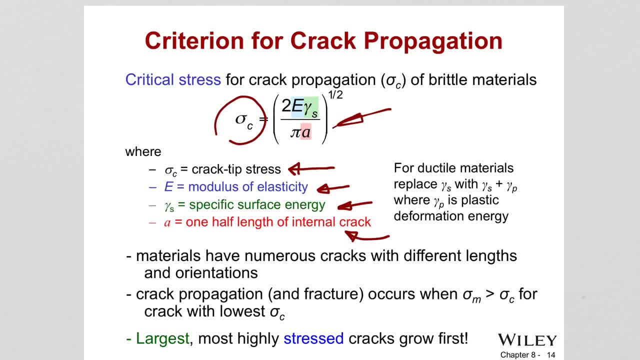 Stress To Propagate, Because It Is Easier To Reach That By Looking At The Equation And Giving A High Volume Right, Largest And Most Highly. 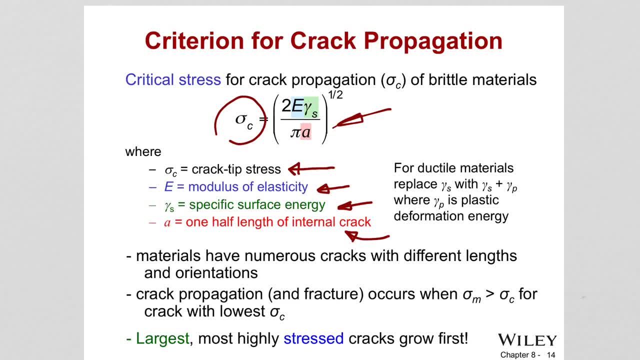 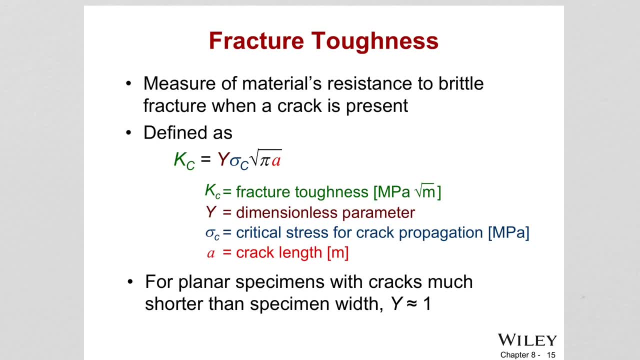 Stressed Cracks Will Grow First. That's What We Can Conclude. So We Have Seen Toughness Of Material Till It Fails Right. Elastic Under. 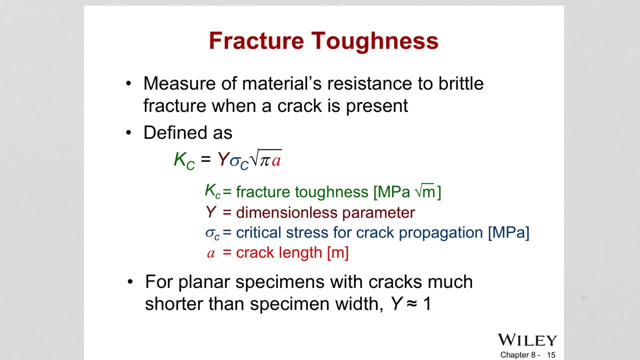 Elastic Region, It Was Resilience, But Elastic Plastic Region. In Total We Called It Toughness. It Was The Amount Of Energy, Because All Materials 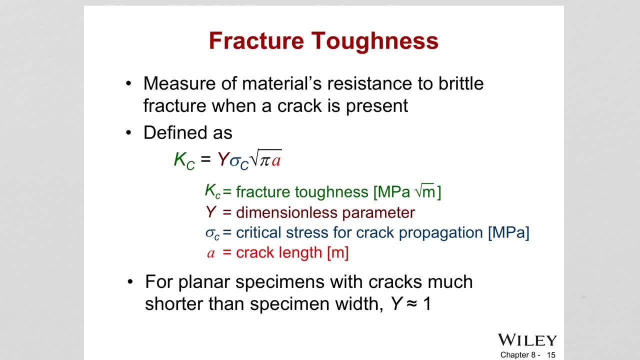 Have Cracks. There's Always A Crack And This Will Measure Us The Resistance Of The Material To Brittle Fracture When A Crack Is. 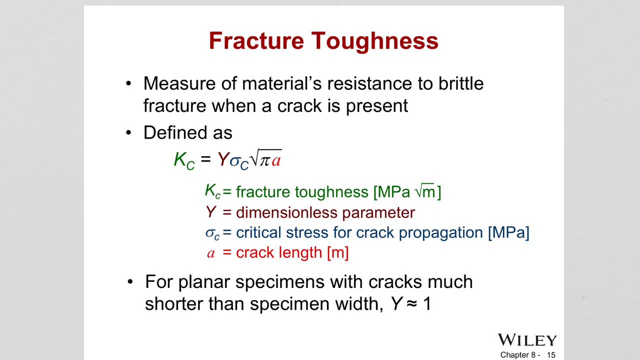 Present. This Is Different Fractured Toughness Volumes And It Helps Us To Characterize Them Based On That. So The Equation To Define Fractured 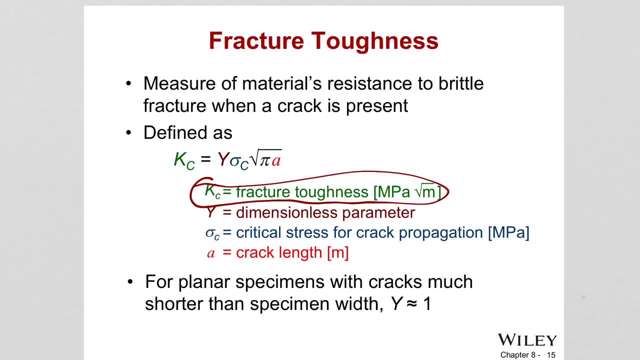 Toughness. It Is Shown With A, K, The C, Y, Which Is A Parameter Based On The Crack And Space Specimen Sizes Geometries. 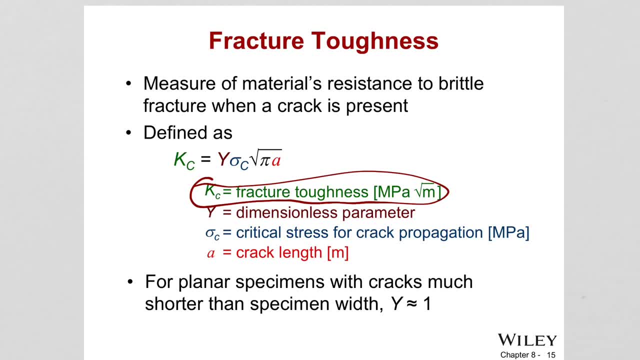 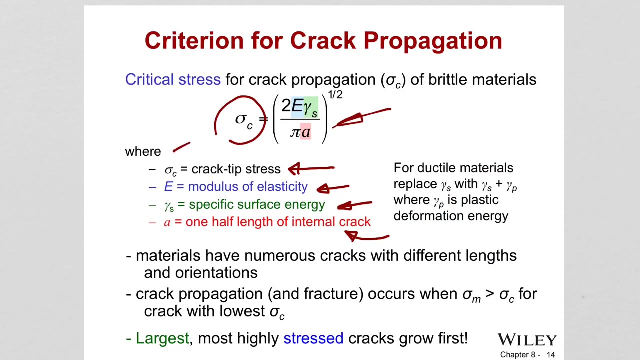 As Well As The Manner Of The Load Applied And The Most Materials We Accepted As One. So Sigma C Is The Critical Stress For 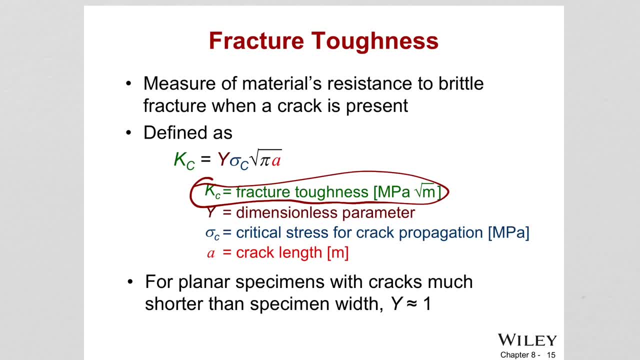 Crack Propagation Here We Learned It Right. So We Learned There Will Be A Stress As The Fractured Toughness Of The Material Increases. For 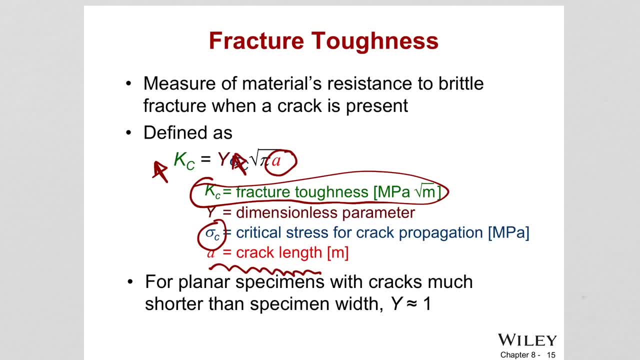 A Certain Crack Size. If We Keep It Constant, The Critical Crack Stress Required For The Propagation Will Also Increase. Look At The Equation And. 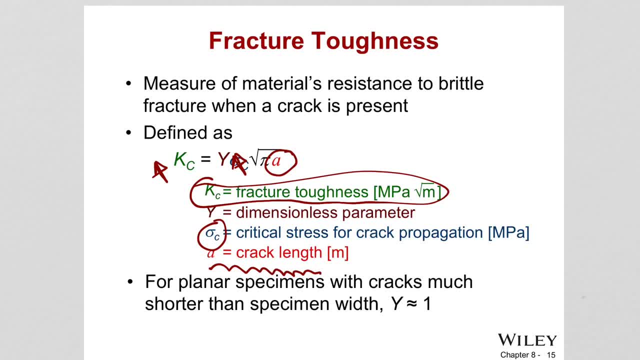 Try To Understand What Is Fractured Toughness For A Certain Size Of Crack A. Basically It Is The Stress Right. Fractured Toughness Is: 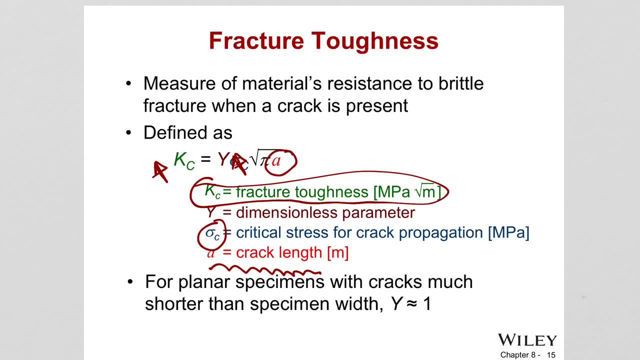 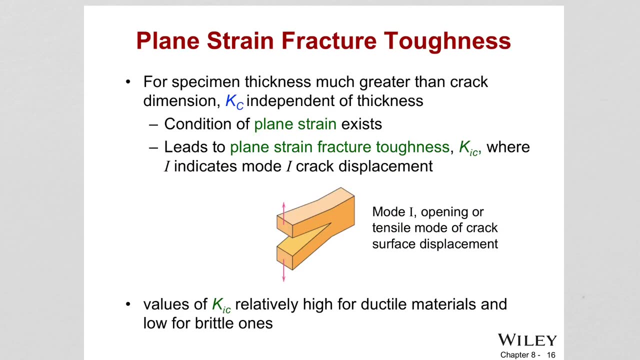 Basically Better Idea Of The Amount Of Stress That Needs To Be Applied, So That We Don't. We Material Will Not Fail By The Brittle. 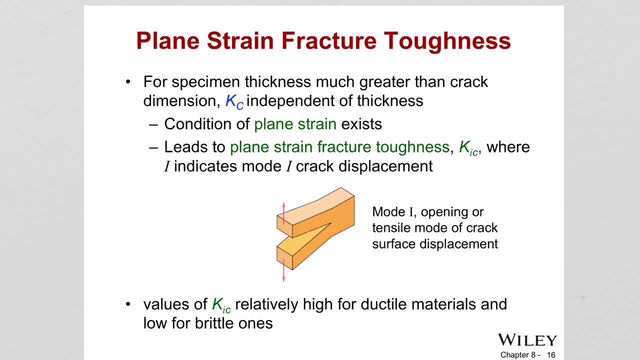 Fracture. So When The Specimen Thickness Is Independent Of The Specimen Thickness, Under These Conditions A Condition Of Plain Strain Exists. What Does 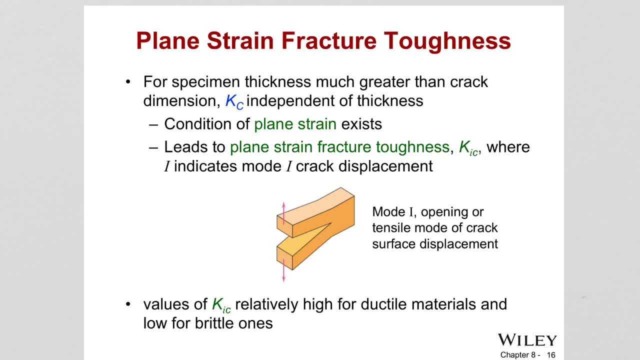 What Does It Mean? Plain Strain Right, So Plain Strain. Basically Deep Changes Of A Material Happen On A Single Plain. In Other Words: 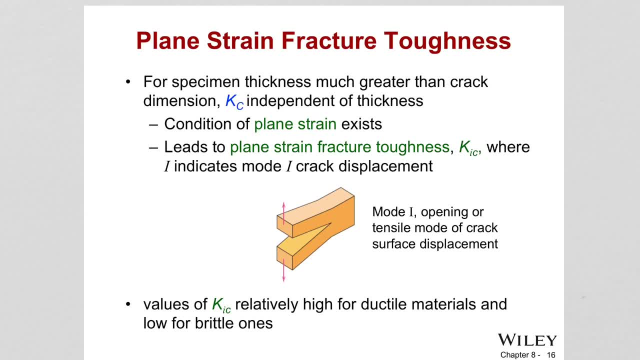 Basically, Displacement Of Material Happens In A Direction That Is Parallel To A Given Plain. So If This Right In The Material We Apply, The 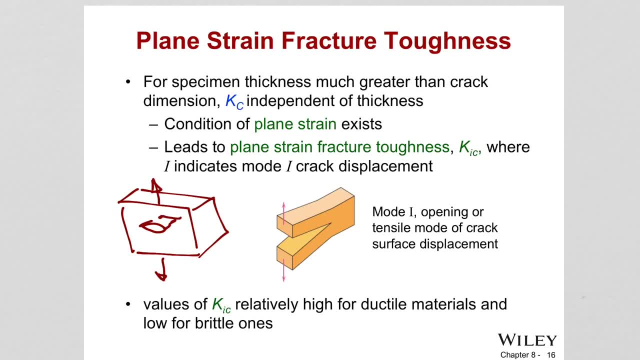 Tensile Stresses Right Deformation, Displacement Will Happen In A Direction That Is Parallel To The Given Plain. So If This Is Parallel To 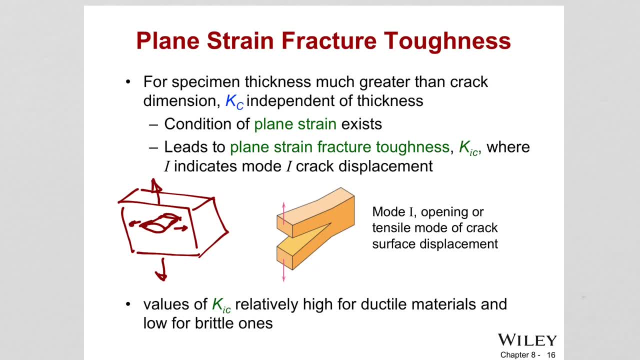 That So That Means The Plain Strain Means There Is No Strain Component Perpendicular The To The Front And Back Faces Of The Crack. 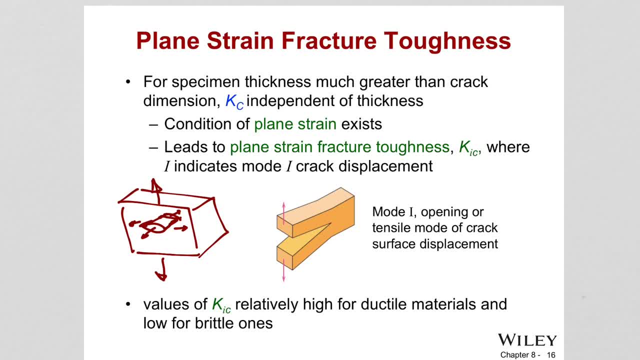 Like This. So You For Then Thick Specimens Known As A Plain Strain, Fracture Toughness, Which Is K, I, C, Here The I. 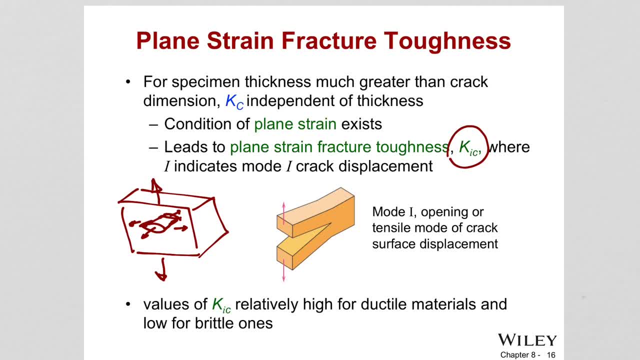 Means Mode I Crack Displacement, Which Happens As You See, Of Crack Surface Displacement, Like We See In The Figure. Well, It Is Defined. 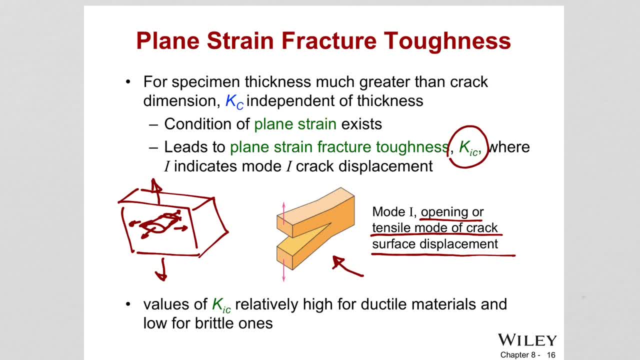 By The Same Equation. It Is Just Telling Us That The This Time We Are Working With, The Crack Is Opening Up In This Configuration. 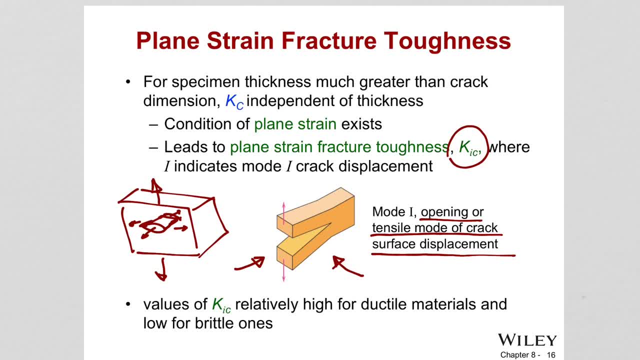 Basically And Of Course The K I C Volumes Are High For Ductal Materials Because We Understood From The Equation Materials, But Lower For. 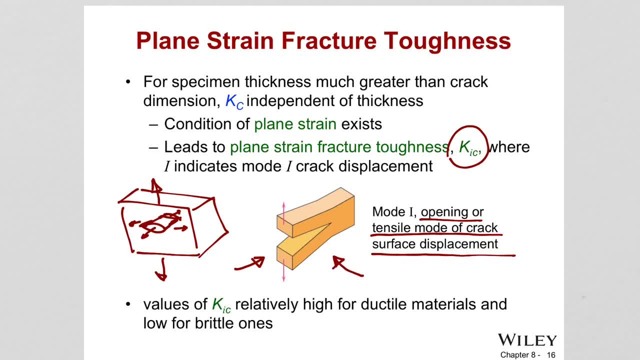 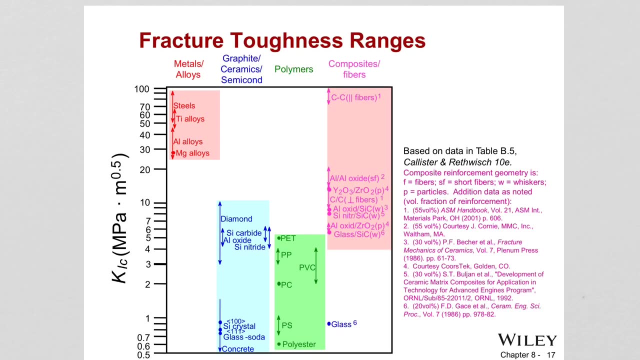 Brittle Ones Though. So We Say The Plain Fracture Top, Plain Strain Fracture. Toughness For Ceramic Is Our Low For Example, Compared. 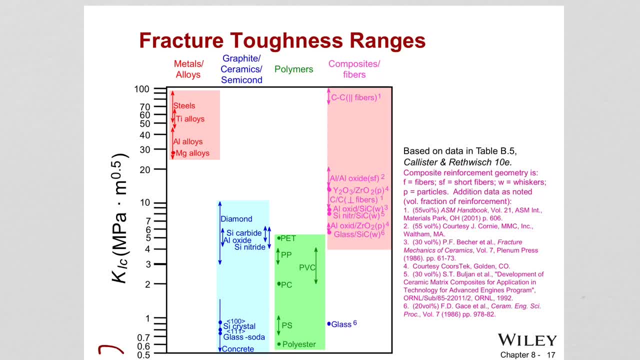 To Metals. So Therefore, As You Can See, Metals And Alloys Has The Highest Volumes Of Fracture Toughness. They Will Require Higher Stress. 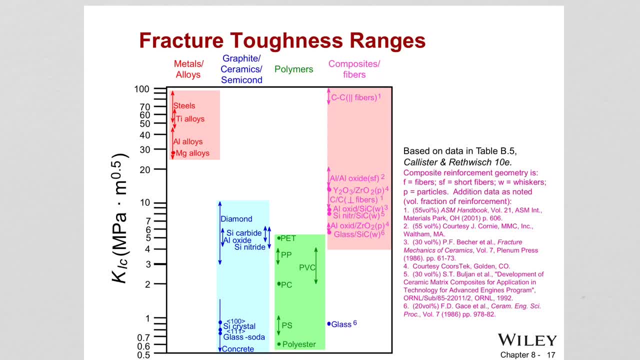 Levels For Cracks To Propagate Where, As We See That, So They Are More Brittle And Composites And Fibers. This Since Composites Are. 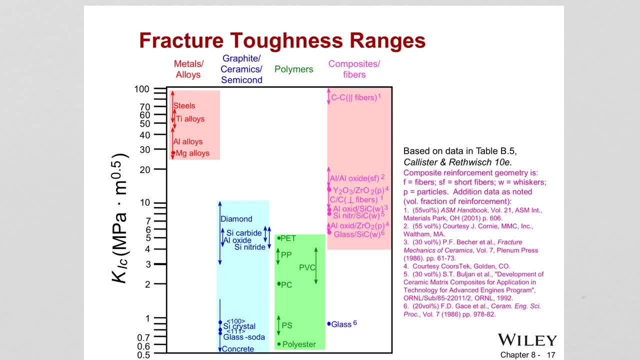 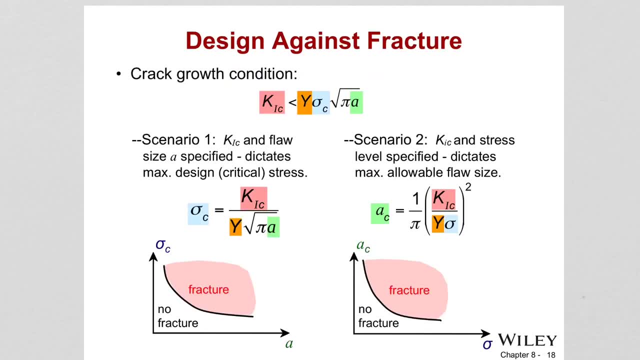 Mixture Of Different Types Of Materials, So In This Case A Wide Range Of Fracture Toughness In Condition Where The Crack Will Grow. We 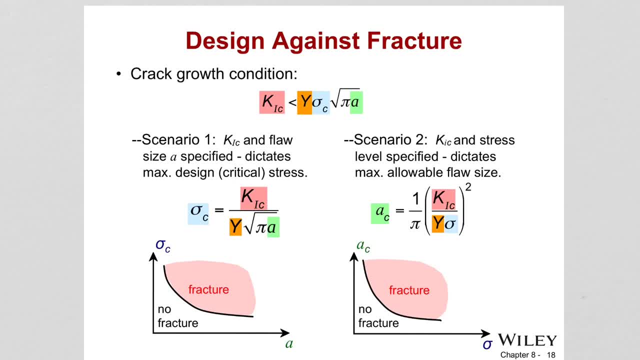 Can Say If, With Given Critical Stress Levels, With A Certain Size Of Crack, If The Toughness Required Fracture. Toughness Required Is Fracture. 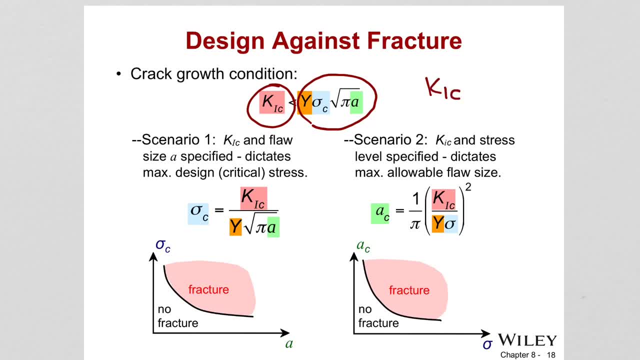 Toughness, The Plain Strain Fracture Toughness. Assuming Y Is One, Let's Delete This, Or Never Mind Y Sigma Pi A. So Now This: 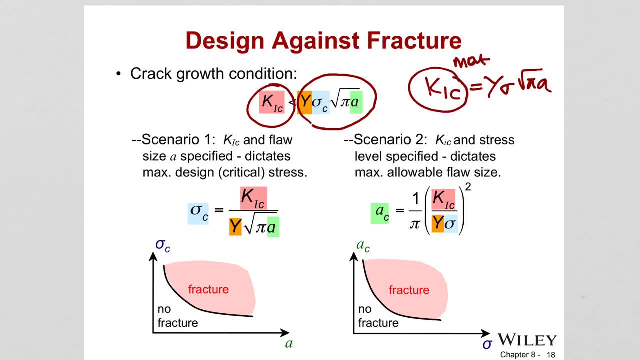 Volume Is A Material Constant So Depending On The Material, It Will Have A Certain Volume, And You Can Find These From Tables In Your Book. 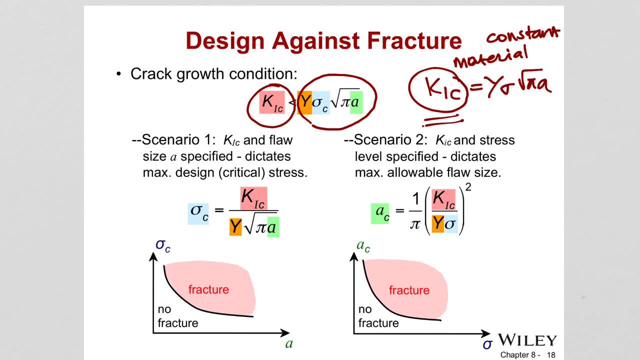 For Example, There Is Table Eight One Which Gives. So If You Know The Fractured Toughness And The Size Of The Crack Inside The 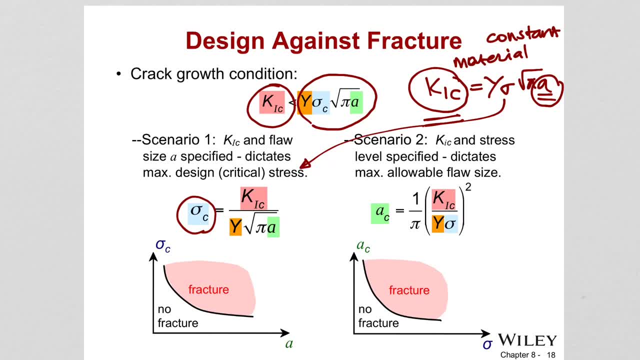 Material. If You Plug That Information In, What You Can Calculate Is Actually The Material. So In This Case You Know K One C, Specific To 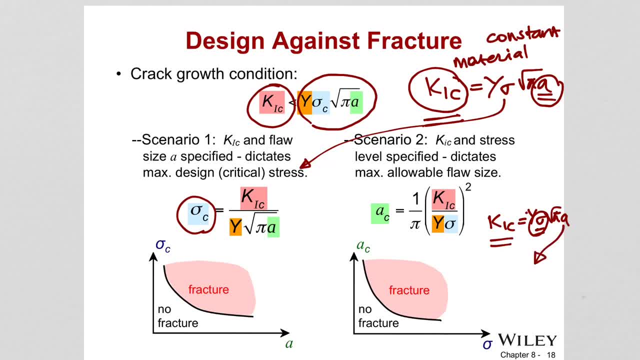 The Material And You Know The Stress That Is Gonna Be Applied To The Material, Then It You Can Find Two Things You Can Find. 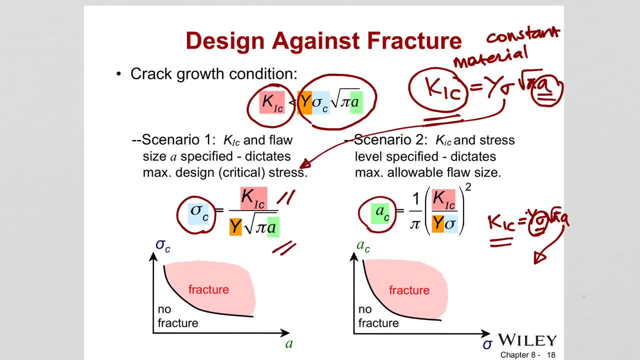 For A Certain Size Of Flow And Fractured Toughness Of A Material, You Can Find The Critical Stress That Is Necessary For Your Material. 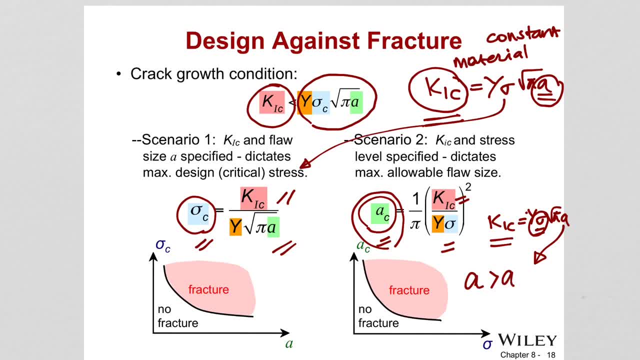 There Are Cracks That Are Bigger Than The Critical Crack Length. They, Already Filled, Met The Condition Of Crack Propagation. Therefore, Your Material, The 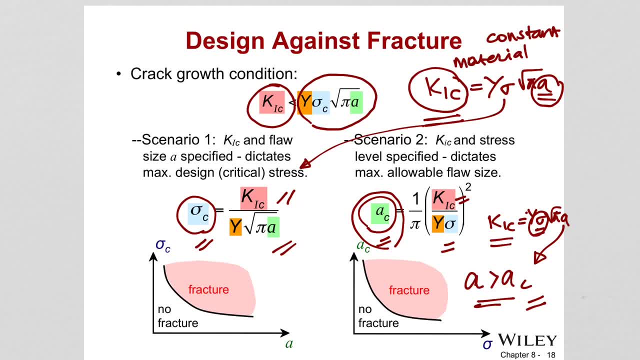 Crack Inside Your Material They Gonna Propagate, Or They For A Certain Crack Size. They Should Never Reach That Critical Stress Levels, Because Otherwise The 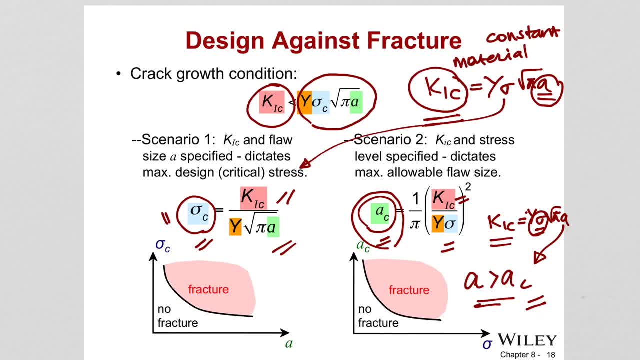 Material Will Fail. So People They Have Developed Loves. This Way They Can Make Sure The Material Is Not Gonna Fail. So They Are Testing. 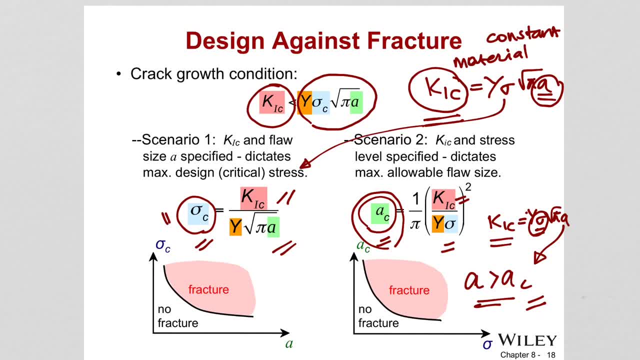 The Aircrafts With These Techniques To See What Are The Crack Sizes. The Same Thing: Right For A Certain Crack Length If You Exceed The. 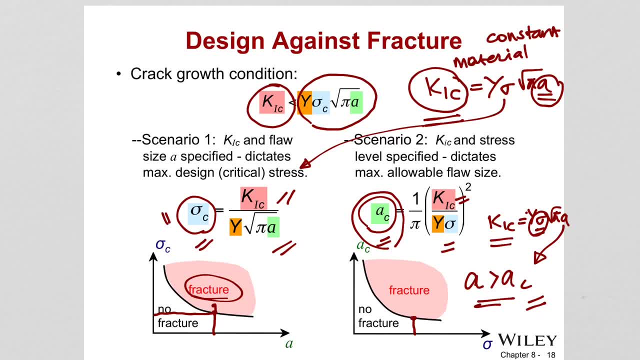 Volume Of Critical Stress, Then The Fracture Will Happen. Or For A Certain Stress Volume, If You Lower The Applied Stress, The Critical Crack 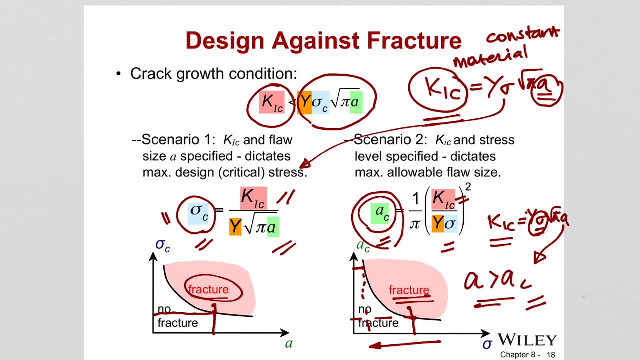 Length Will Increase, You Are Safer And As You, As You Increase The Crack Size, The Critical Stress Level Will Decrease. Right This Crack Propagation. 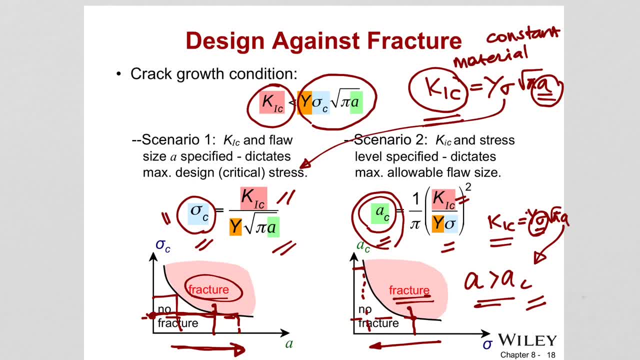 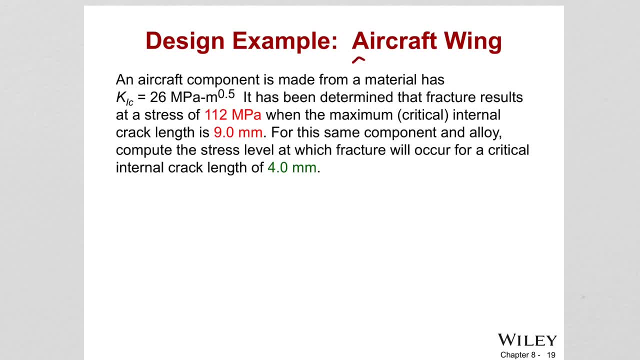 With Will Decrease. So Design Example For An Aircraft: Wing. There Is An Aircraft Made From A Material That As Reno- Yeah, There Is a Fracture. 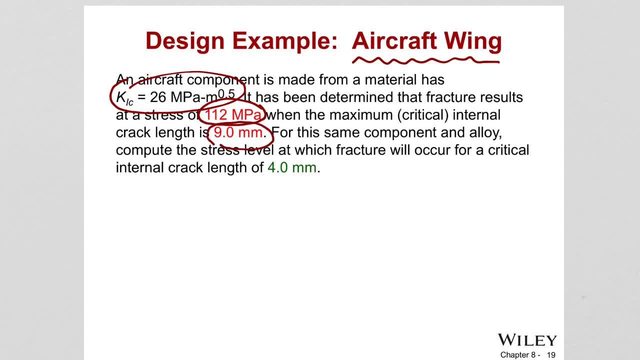 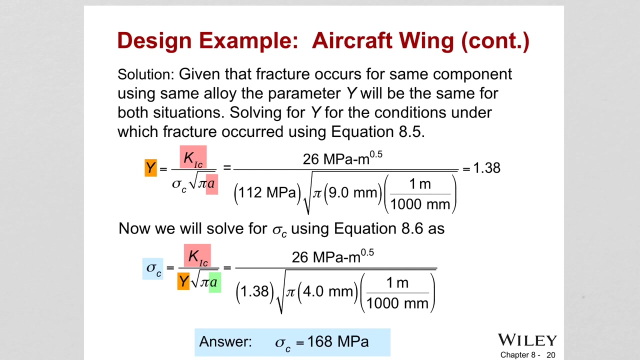 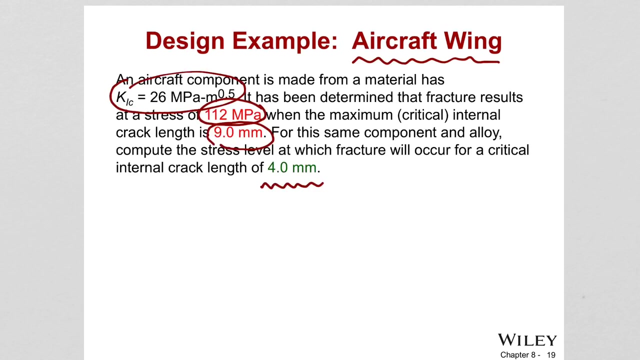 It Is The Critical Integral Crack Length Of Three Millimeters. Now We Have Been Given A Most Important Factor In A Aircraft In Material, the conditions of, first of all, we are given the fracture toughness and we are given the 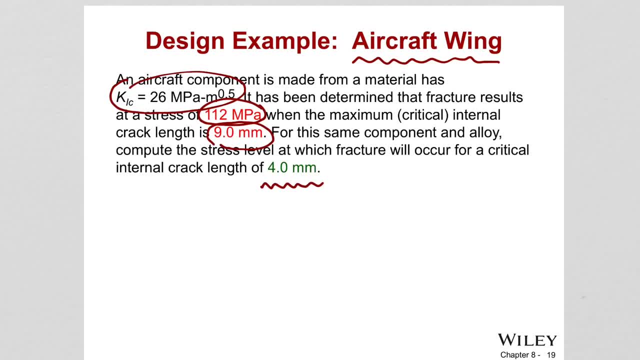 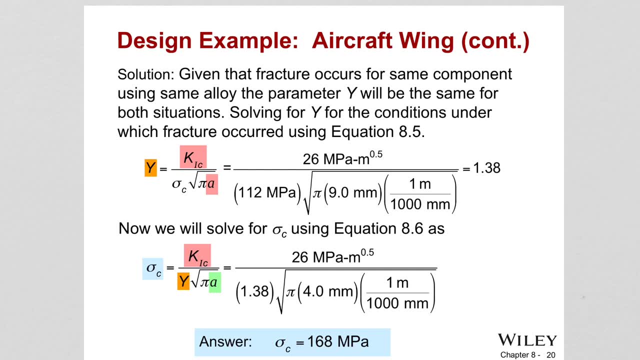 critical stress that is happening at that critical crack length. so plug in the information into our equation. what we gonna find out. so this was the fractures toughness, this is the a. of course, be careful with the units right. this is the a and then this is the critical stress. so with those, 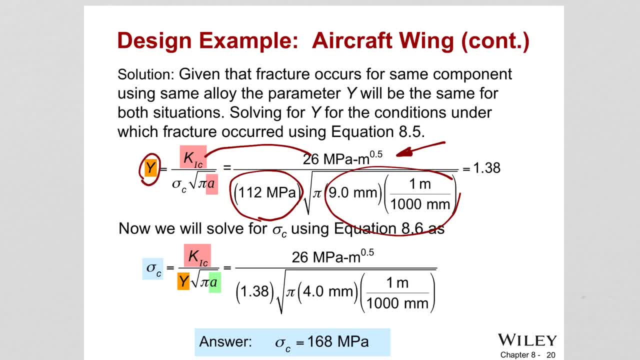 conditions, the y. the constant parameter is one point three eight. now, once you find that why, you can use it again, because it will be the same for the same condition, same material. you can use that constant again to find the critical stress for a crack length of four millimeter. now you're. 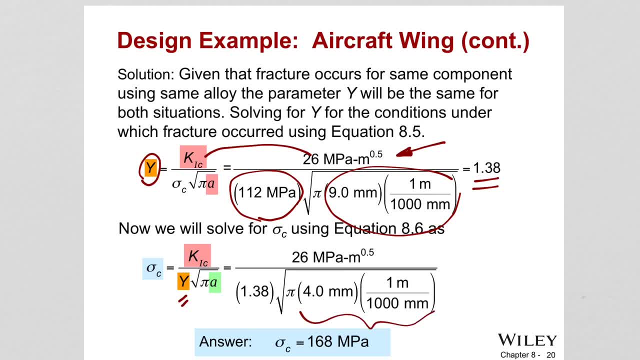 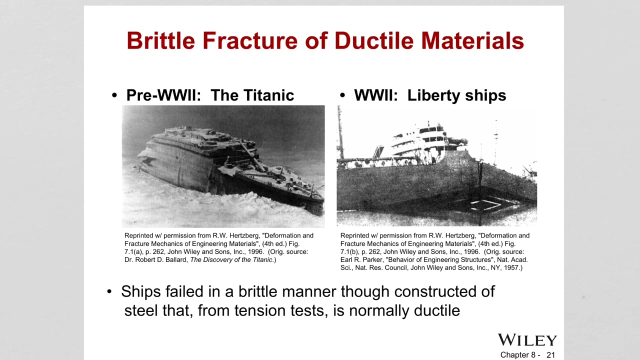 going to put the four here. the correct size, here the fracture toughness is the same, because same material. why is the same same material? and then for that correct size, your critical stress stress is 168 MPa, so you should not exceed this volume. So if a material is ductile, it doesn't necessarily mean that it's not gonna fail by brittle fracture. 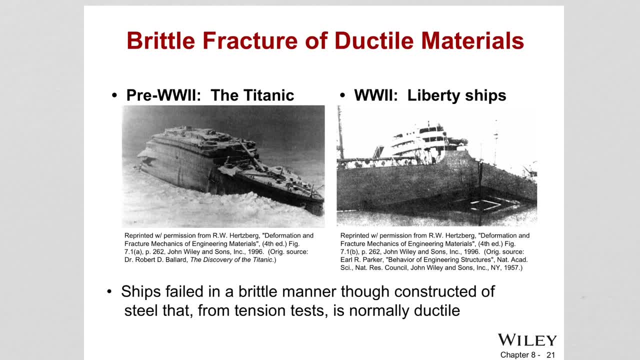 And the obvious examples of those are Titanic and World War II Liberty ships. What happened, as you can see? sudden fracture, failure. And for the Titanic it is the same. So normally they are made out of steel, which is assumed to be, which was assumed to be. 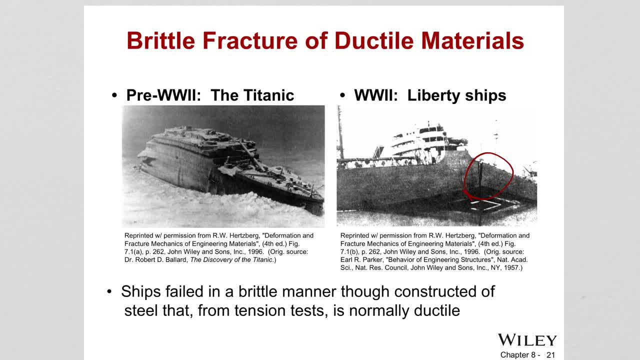 very ductile, very strong materials which can handle anything. But what happened, What happened here, is these materials failed with a brittle fracture. And why this happened? The same as the Challenger disaster: Normally ductile material, which was rubber, failed with a brittle fracture. 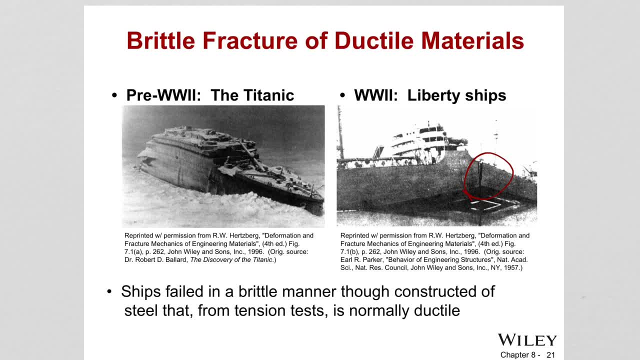 So why is this happening? It is because the normally ductile steel will behave as a brittle material When we go below certain temperatures. So in summary, we can say that the temperatures are affecting the behavior, therefore the failure of materials. So they, on the Titanic case, they were going on the cold waters, right. 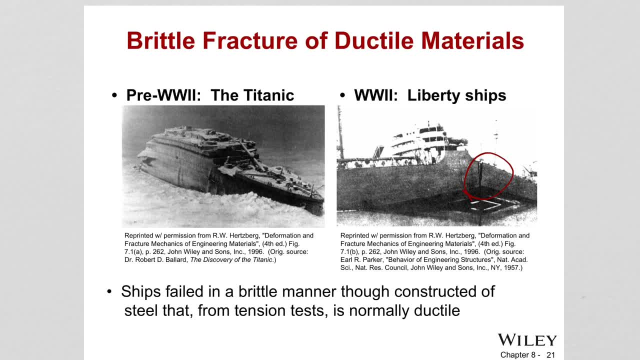 They hit the iceberg. It was cold waters, And the normally ductile steel at low temperatures behaved as a brittle material. Same happened for the Liberty ships World War II. They noticed only the ships that were exposed to cold temperatures- sea, ocean temperatures. 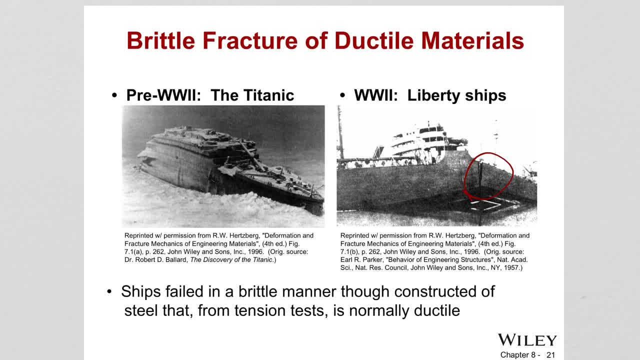 or experiencing failures, such, such, such sudden failures. And then what happened in the Challenger disaster is the date of the launch, The temperature of the ship, The temperature of the ship. The temperatures were minus four, So normally the ductile rubber behaved as a brittle material and failed suddenly, couldn't. 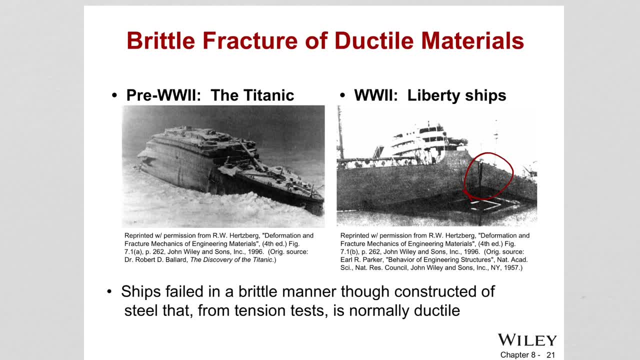 see, couldn't perform its sealing functionality. So therefore you guys need to be careful at what temperatures these materials are you are going to be used, because that will directly determine the failure mechanisms of those materials. So then we can say that, uh, how the material will fails actually depend on the temperature. 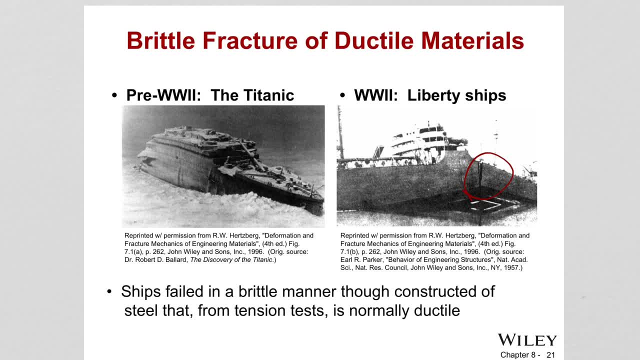 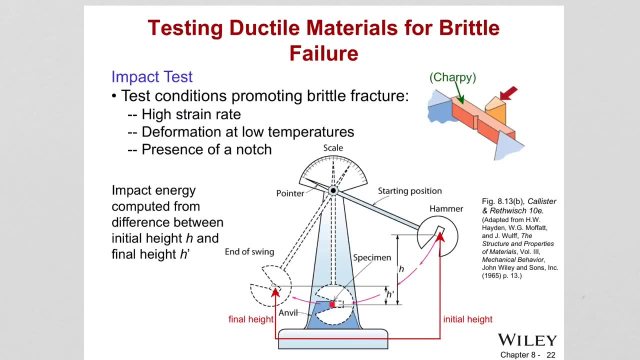 And there is a temperature where the material uh changes behavior from ductile to brittle. So how do we test materials Then for this brittle fracture? How do we test materials fracture? and we have the Charpy impact test which measures this behavior of 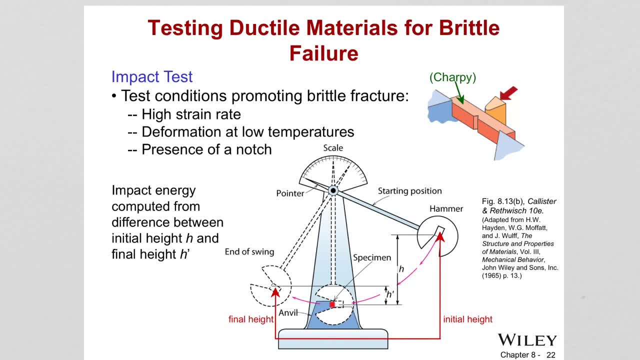 materials. so here, first, I suggest you guys don't forget to watch the video links, videos I am sending you from canvas, okay, because you can see there how all these experiments are done visually. in those videos you will also see, depending on the fracture surface, how people can. 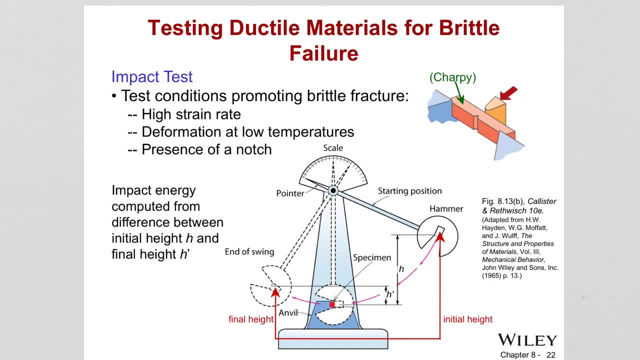 characterize if it is a brittle or ductile failure. so for a ductile material, this sample is prepared with a notch okay, as you can see. and then brittle failure: the brittle fracture conditions are promoted, such as high strength율 for Caravel joining and doit raw material for to large. kijkenp enables ship measures and many more. 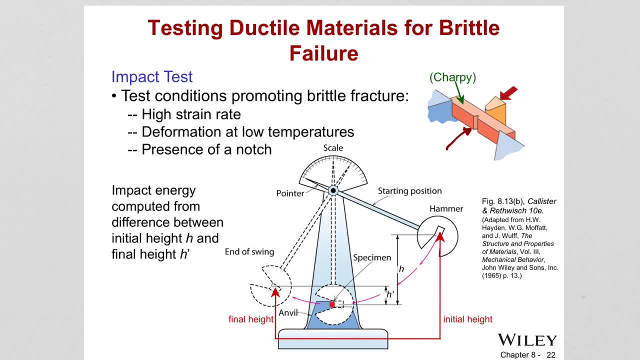 strain rate, deformation at low temperature and the presence of a notch. So what is done is basically the energy absorbed for this crack to propagate is calculated How There is a hammer. So there is your specimen here, right there, And there is the hammer. 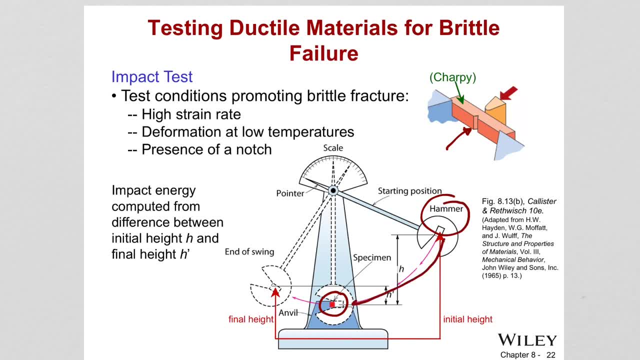 At a certain height, which hits, released and hits your material. your material breaks and then the hammer continues its journey and comes to this position, now at a different height. So its potential energy changed and this change in energy is actually the energy absorbed. 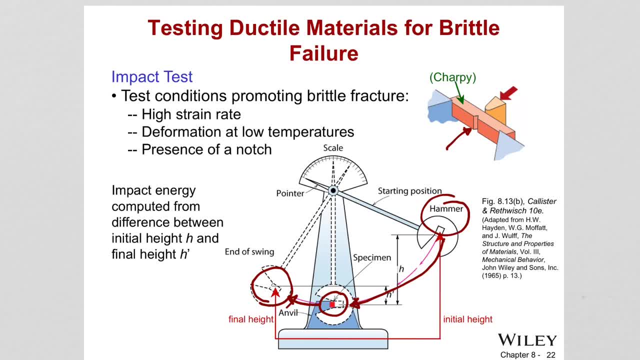 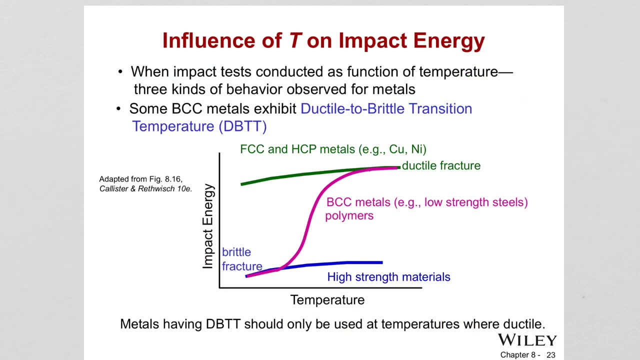 by the material energy absorbed for that crack to propagate and fill the material. This is what we call as Charpy test. So what about? as I said, the temperature has a great effect on the impact energy, So whether the material will behave as brittle or ductile right. 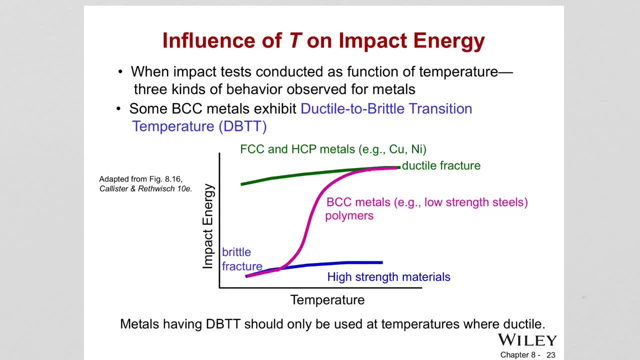 Higher impact energy means material absorbed more Right. The material absorbed more energy before it fails. Low impact energy means material didn't go through any plastic deformation anything to absorb those energies and it failed suddenly with brittle fracture. So as a function of time for different types of materials, people calculated the impact. 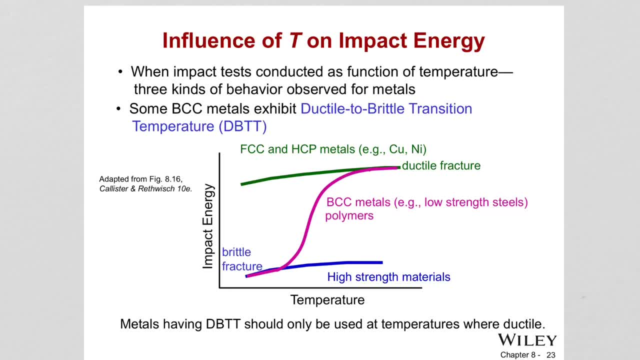 energy of those materials with a Charpy test And then they put it on a chart. Okay, that is what we are seeing here. Three types of behavior is observed. Either materials cover completely ductile throughout every temperature, throughout the increasing temperature- here with the shown with the green- or they actually change behavior. 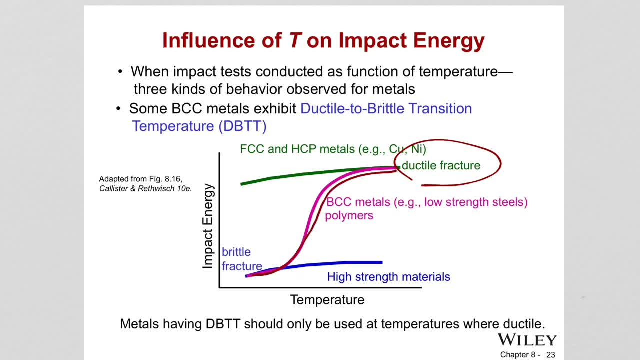 from brittle, For example, if the material gets exposed to the ductile high impact energies, from low impact energies to high impact energies at a certain temperature, or they will always stay like a brittle material throughout the temperatures. So this was found to be related to the structure of the materials. 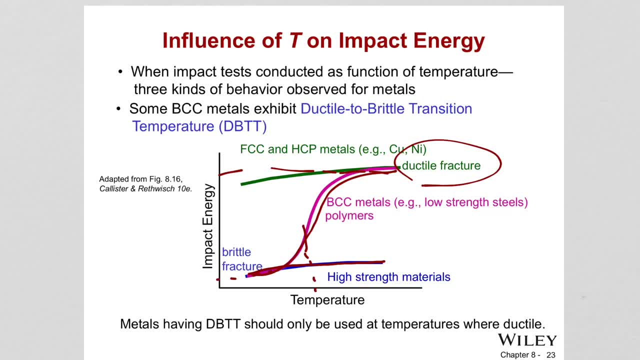 The structure should be related to the structure of the materials. So for FCC and HCP metals such as copper, nickel, these materials are ductile and these materials behave as a ductile as we increase the temperature and it doesn't change behavior with changing temperature. 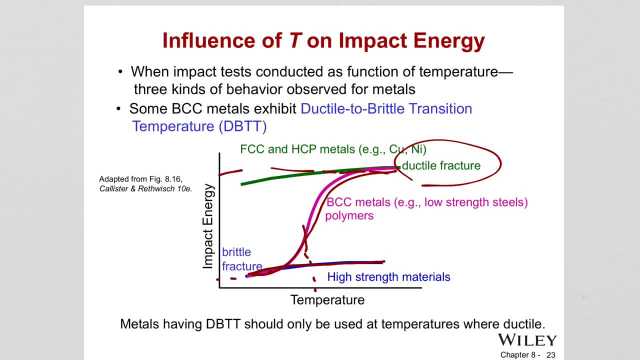 But BCC metals. they experience a change from a bridal fracture to ductile fracture, as you see with the pink, And the temperature is usually taken in the middle of this range. this change range and read as the ductile to bridal transition temperature: dBTd. 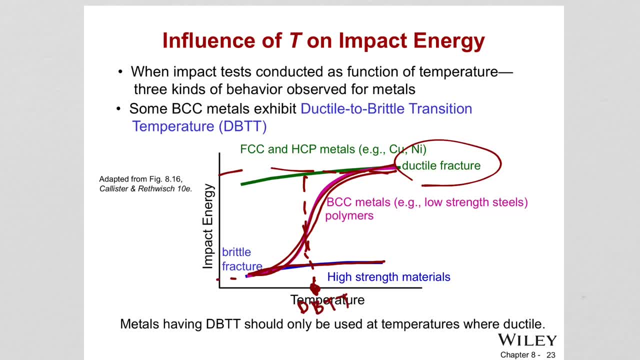 Okay, So for high strength metals they always behave as bridal. It doesn't matter what temperature it is, And we know the higher the strength, more bridal the material. So we know that. So if you are using a metal in your manufacturing of your parts, 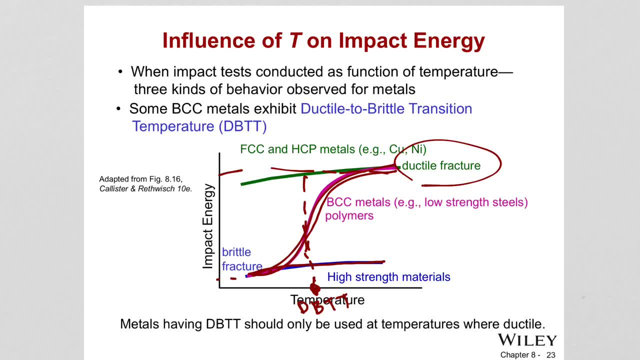 you need to be careful because at what temperatures you're going to use them? you don't want to go below the ductile to brittle transition temperature, where the behavior of the material is not brittle. this is the reason why they made mistakes and for the titanic and then liberty ships. 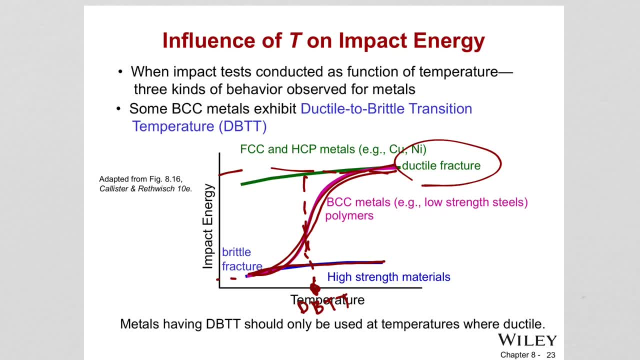 they chose. they didn't take into account that the behavior of materials can change with the temperature, but in fact it was changing. they were using steel, and that is bcc, and this was therefore their behavior, dependent on the temperature. so the difference we are seeing here between fcc- bcc is related to the packing. so we know. 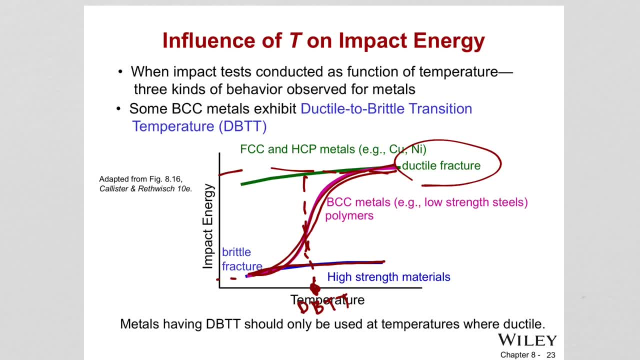 fcc, hcp are more densely packed structures compared to bcc, and then there will be several planes and direction where the deformation can take place. but, of course, hcp metals are not going to be as ductile as fcc metals because number of slip systems were much lower, if you remember, and there are other factors affecting bcc metals, such as 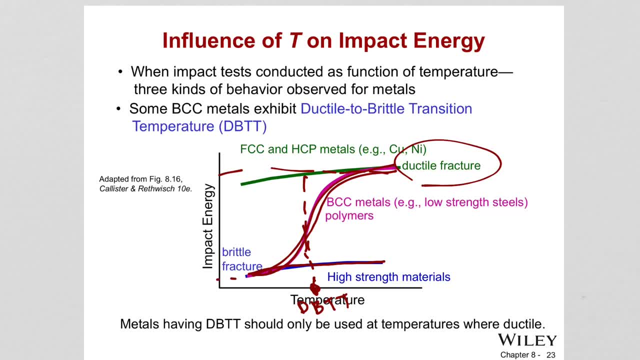 steels, like the alloying the presence of carbon. those type of alloying elements can also affect the bcc metals and the bcc metals. can also affect the bcc metals and the bcc metals. the behavior of materials based on depending on the temperature as a function of temperature. 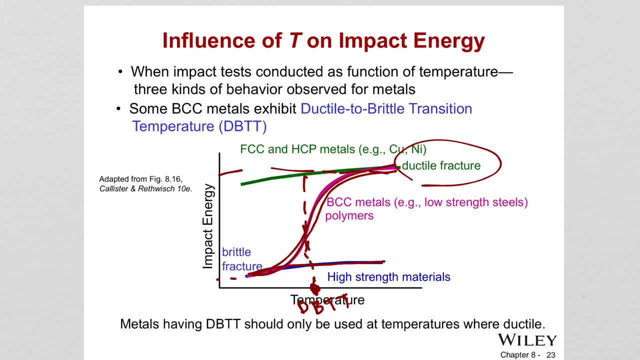 so therefore this is generalized behavior. but then for each material that you are working with, specific material, you need to calculate the impact energy as a function of temperature. then, based on that observation, you should go ahead and choose that material for your application. make sure that you never go below that ductile to brittle transition temperature. 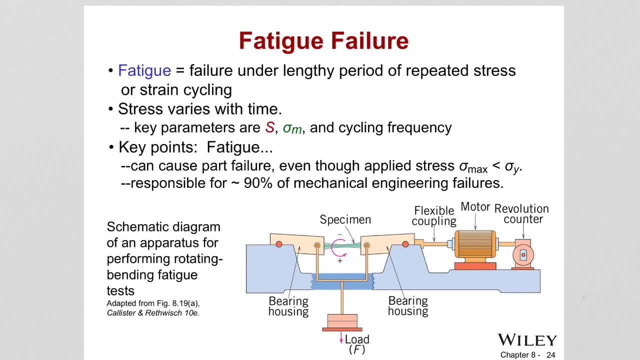 so fatigue, failure. what is fatigue? basically, if you expose the material to repeated cycles of stresses, then with time the failure will happen. there will be a crack and the formation and this crack will propagate. so stress cycle means many of the parts that we used in applications. they are exposed to stress cycles like tension compression. 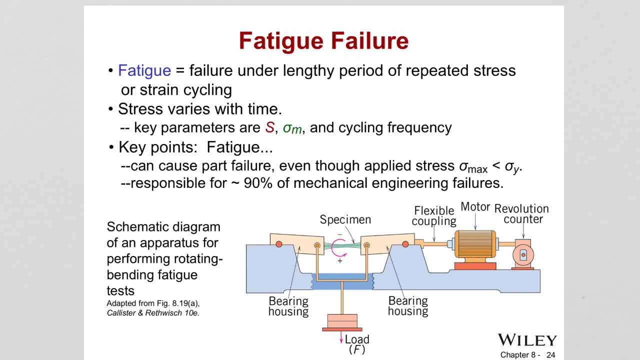 tension, compression, or bending twisting, bending twisting. so there is just this cycle going on. for example, we can say: stress is on the y-axis, time on the x-axis. this positive stress are representing tension, negative stress, stress values representing compression. the material is exposed to tension, then compression. 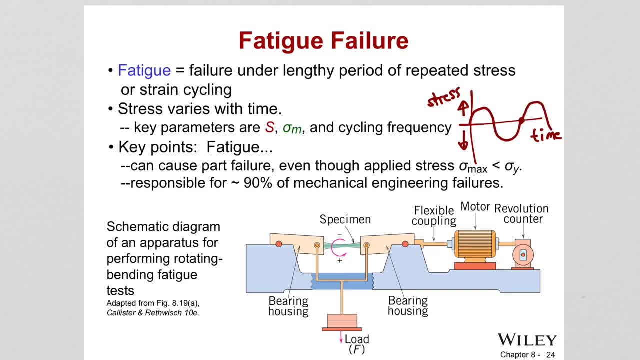 completing one cycle, tension and compression completing another cycle. so each cycle of stress strain, i mean each cycle of tension and compression, right with time. if the material exposed to these cycling stresses, with time, cracks can form and propagate in the structure, so this represent the maximum stress tension stressed material is exposed to. this is the 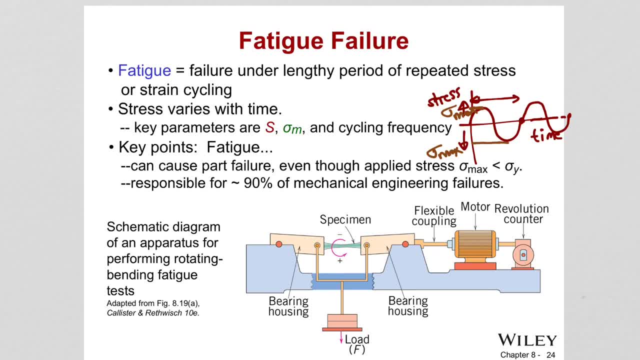 maximum compression stresses the material are exposed to, or we can say here minimum stresses anyhow. okay, so then we understand that the stress varies with time and the parameters are the applied stress and the mean volume of stresses. so the mean volume is the mean volume of this each cycle. so maybe 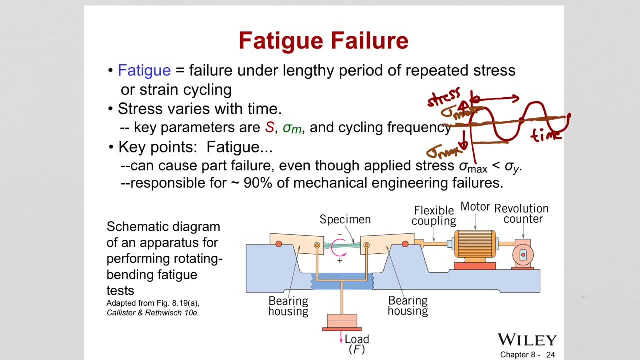 of course, here it is right there. if it's symmetric and this is a consequence like this there, this is okay. it doesn't have to be symmetric. it can be like more tension than compression, right? so it can be like this. then, if there it is the case, you need to find out- mean, will you in between these? okay? 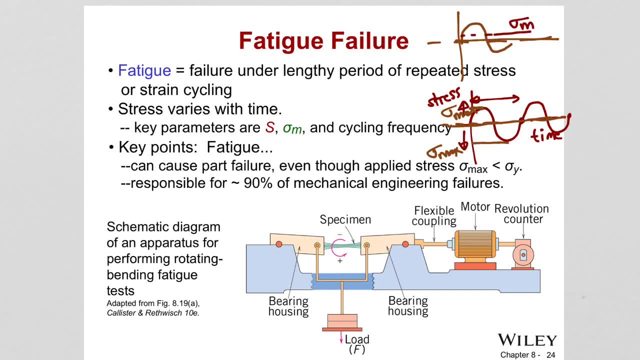 something like, somewhere like this. so it is important to understand and that ARE CAUTION FACT. by미, in your design, you might have chosen your material in a way that the applied stresses are actually much lower than the yield strength of that material, and you might think you are safe. 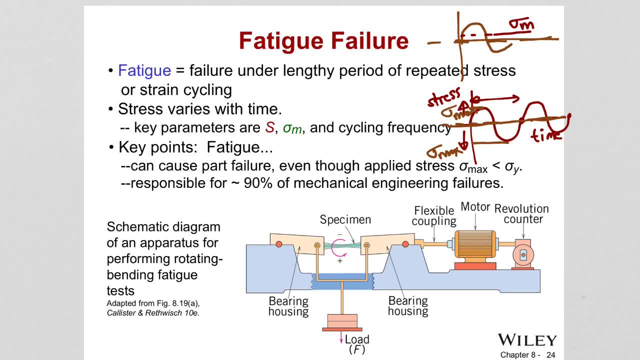 However, the fatigue failure happens when the stress levels are actually much lower than the yield strength of the material, and this is the most common way that materials actually fail, and you can see a schematic of an apparatus for performing rotating and bending fatigue tests. So it is exposing the material to cycles of stresses. 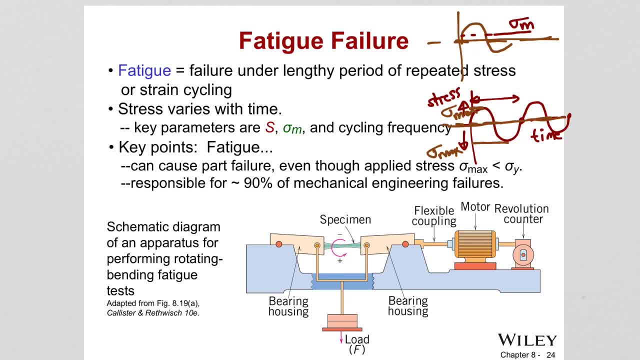 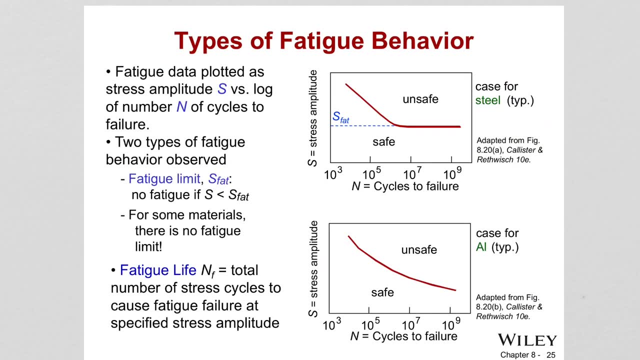 and therefore measuring basically how long it takes the material to fail at certain stress levels. Now, this part is important, right? so what does this test measures? So, first of all, it records And therefore measuring basically how long it takes the material to fail at a certain stress levels. 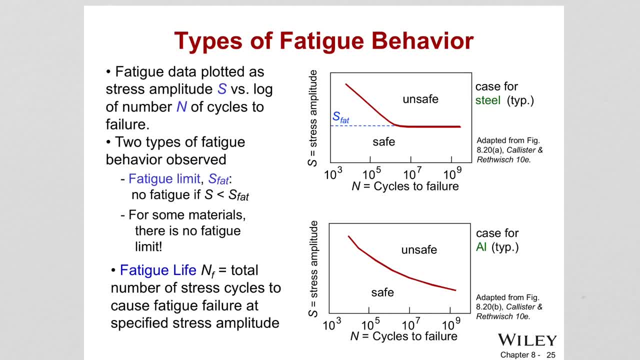 apply stress amplitude as a function of number of cycles to failure. that means at a certain stress level it might take 100 cycles material to fail. remember each cycle is one tension, one compression is a one complete cycle, right, so at what stress levels? uh, it will cause to failure at how many cycles of. 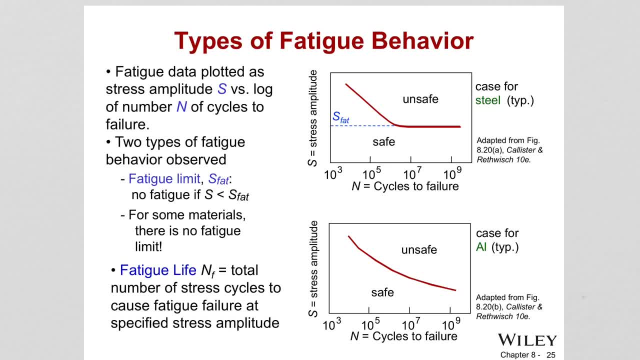 uh, that, repeating uh, stress stresses. so let's say, for example: um, at the certain stress value, it took them 10, to the power of five cycles to experience failure. so based on that, they collect data points right. and then this is how the curve looks like. so, with stress level, with decreasing stress level, stress amplitude, it takes a longer time. 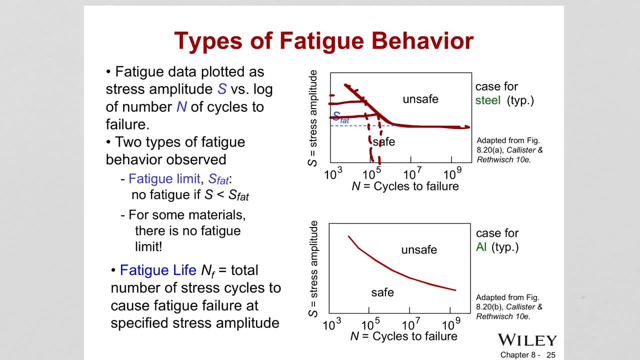 longer amount of cycles for material to fail, but at a certain stress level, which we call the fatigue limit. at a certain stress level, which shown with the blue uh fatigue and under this, if you go under this and if you reach that and go under that stress level, 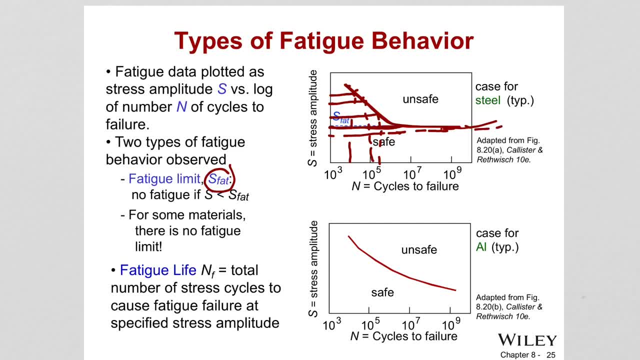 fatigue failure never happens, no matter how many cycles of stress you expose the material to. so that is the fatigue limit. therefore, in your design, to be in on the safe side, you just want to be working below that level of stress. so you just want to be working below that level of stress. so you just want to be working below that level of fatigue. 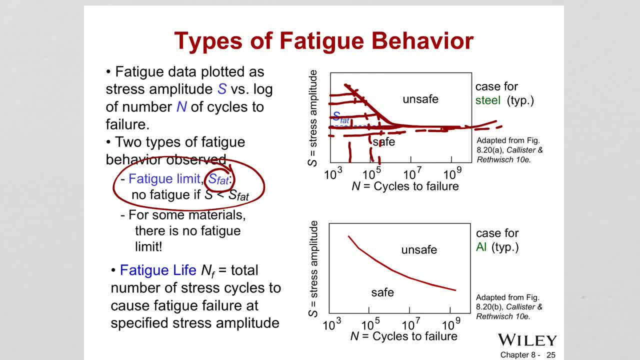 fatigue limit. so actually failure with fatigue never happens when you go below that. all right. for some materials the graph shows differently, such as aluminum, and there is no actually fatigue limit. so you cannot say you can be safe when you have certain number of, when you have a certain body of stress. there is no limit. 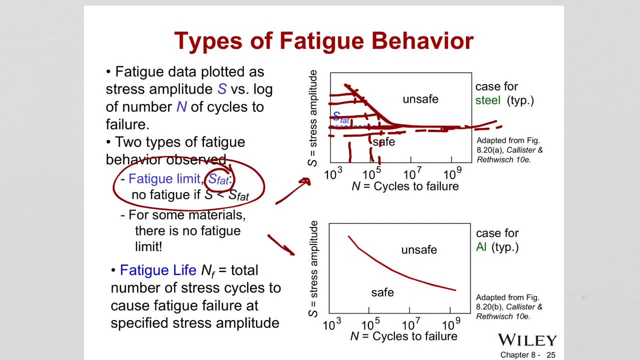 like this one, but it they are, behavior shows up like that, so therefore you need to be careful. at this certain stress level, this much of cycles will cause failure. so, based on this graph now, you can make sure how many cycles the material is going to be exposed to, or one. 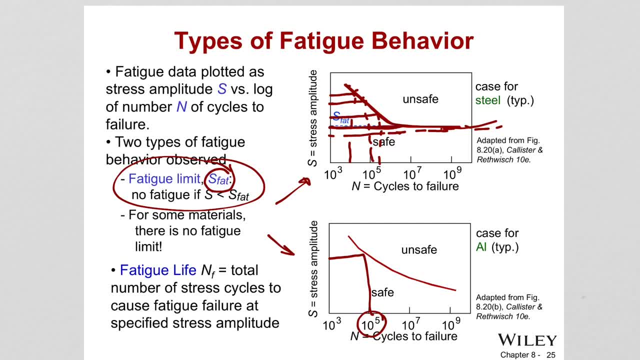 how many cycles the material is going to be exposed to, or one What type of stress level I should be using in order to make sure the material is going to be safe. So NF is the number of cycles to cause the fatigue at a given stress amplitude. 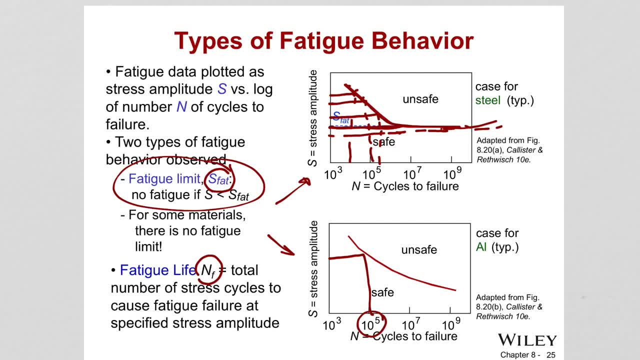 Just like I described. So if you know, if you know, if you did say, if you collected data, you collected data, draw, plot your SN curve for their specific material and then you want to calculate the fatigue life. Of course you know the stress levels that you expose the material to. 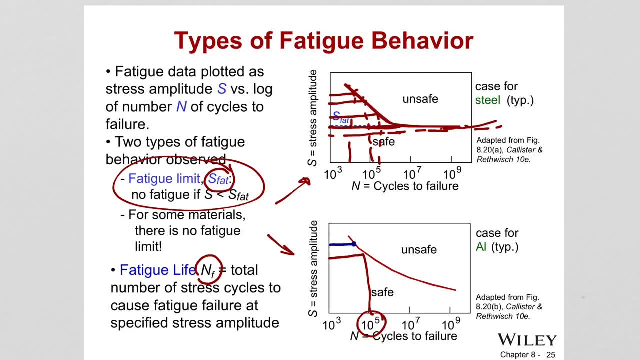 So you go ahead to your chart and find that at stress level, what is going to be the fatigue life, The number of cycles that you can expose the material to, Because when you go above this fatigue life, basically the material will fail at that stress level. 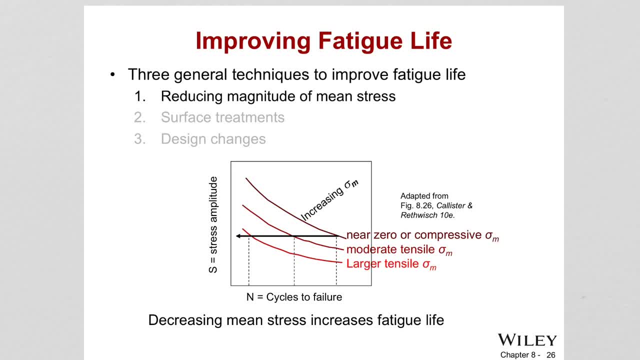 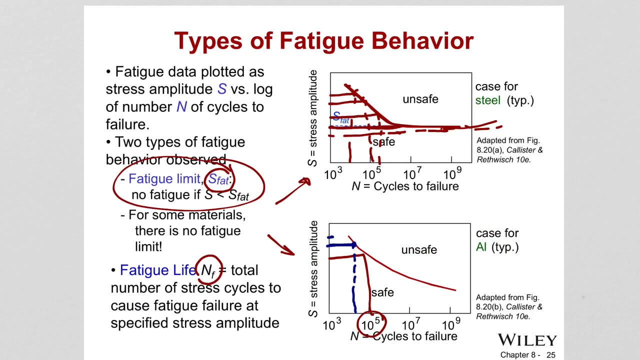 So how can we therefore improve the fatigue life of materials? So what you can do is you can reduce stress. You can apply stresses right. Basically, if you reduce it, if you reduce it, the material can handle more cycles of stress. 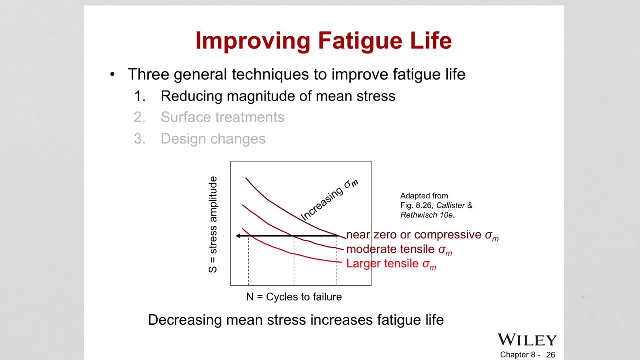 Right, And this is one way of doing it. So we can say: decreasing the mean stress increases the fatigue life. Okay, Okay, Okay, Okay Okay. You are also seeing the effect of a mean stress in the SN curve. you can see that for a certain 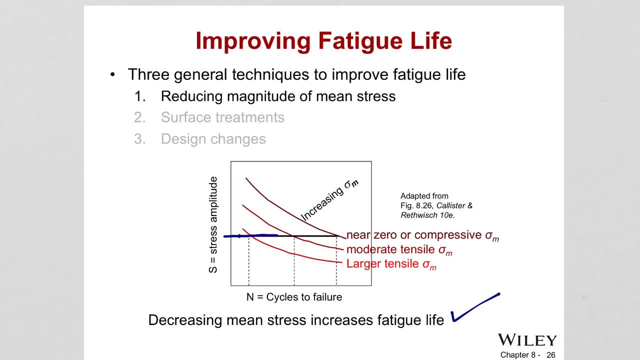 number of stress, certain volume of stress level. if you have larger mean stress levels, number of cycles to failure is lower compared to where you have a more moderate mean stress levels. then you will have a higher NF volume compared to this right. so therefore, this is the summary here: if we 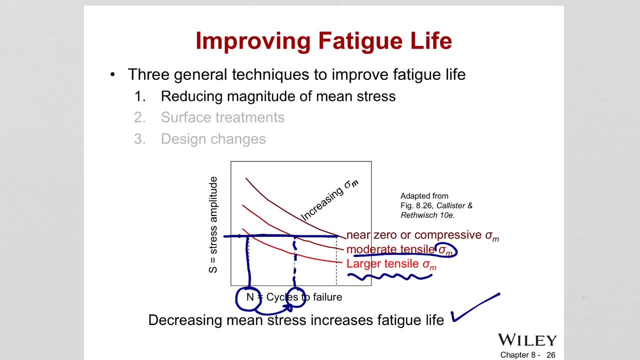 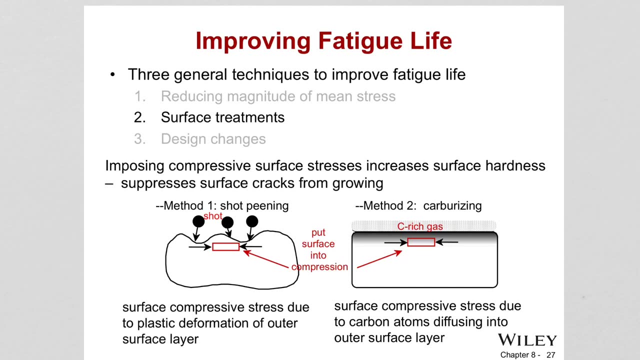 decrease the mean stress, we increase the fatigue life or we increase NF right, the number of cycles to failure is increased. there are other ways, such as doing surface treatments, to increase the fatigue life. so this is some techniques, such as shot, peening or carburizing. so 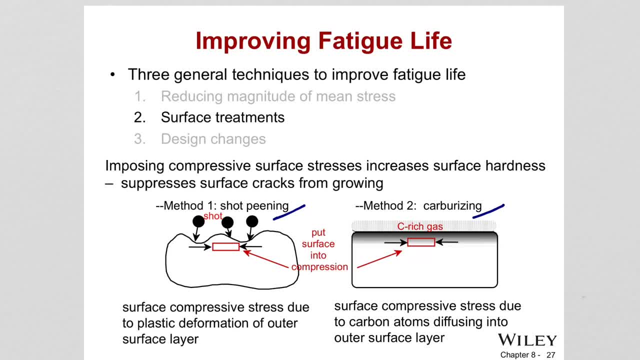 which will strengthen the material. okay. so if you do shot peening, what is seen in the video is that if you do shot peening, what is seen in the video is happening here. you are introducing compressive stresses to the material, the same as carburizing when you expose the material to carbon, rich gas and the 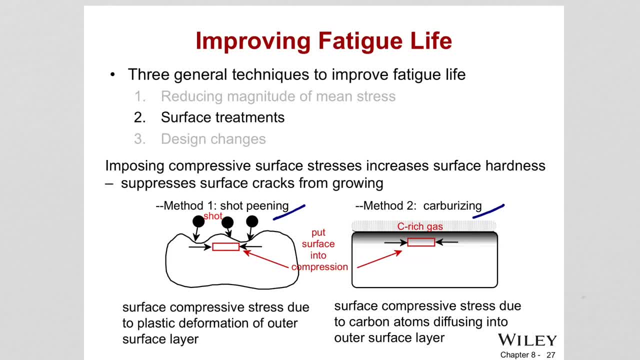 carbon diffuses into the material. so these techniques introduces compressive stresses to the surface of the material. so this is a way to prevent cracks from growing and and if you apply the tensile stresses first, it will need to be compensated by, it will need to get. 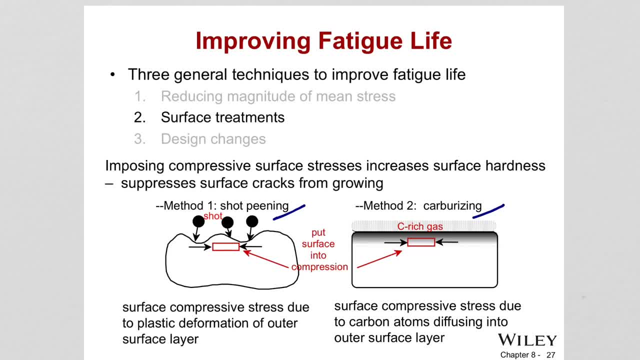 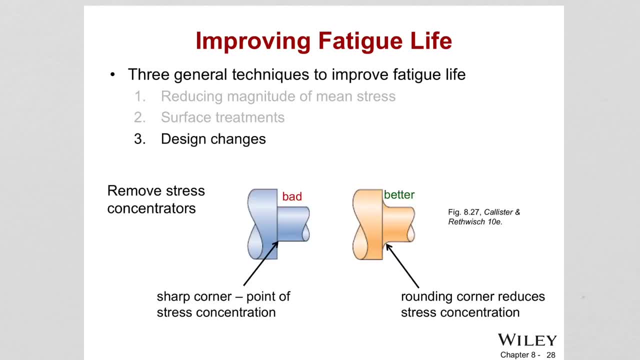 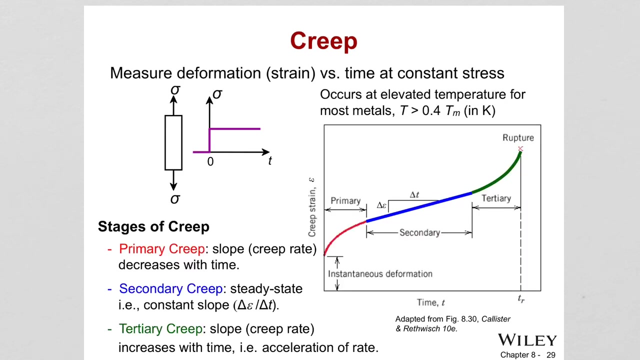 over the volume of that compressive stresses on the surface. and then the design changes, as we said, that we need to avoid those sharp corners to reduce the stress concentration factor, usually happening at elevated temperatures or when the surface is dry. so you usually need to use a 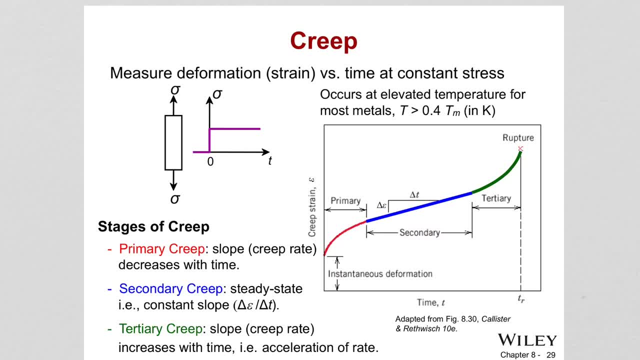 When the material is exposed to static stress at a certain amount of time, at a constant stress level, the material can fail with what we call creep. This is how your tungsten filaments and your light bulbs fail, And there is a life to lifetime that we can give to the light bulbs, right. 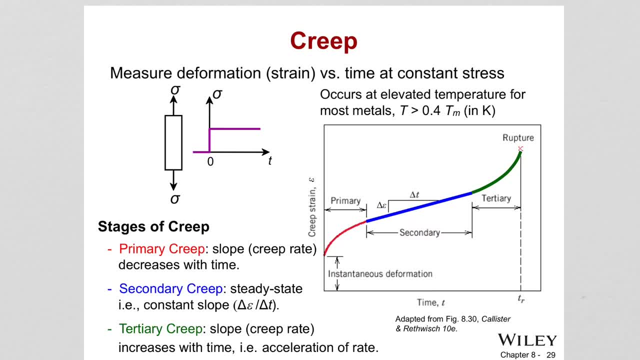 So what happens on those? the tungsten filament sags over time under its own weight, So there is the constant stress which is under its own weight, So very high temperatures in the light bulb. Therefore, with time, that light bulb, actually the constant filament, actually sags and touches each other. 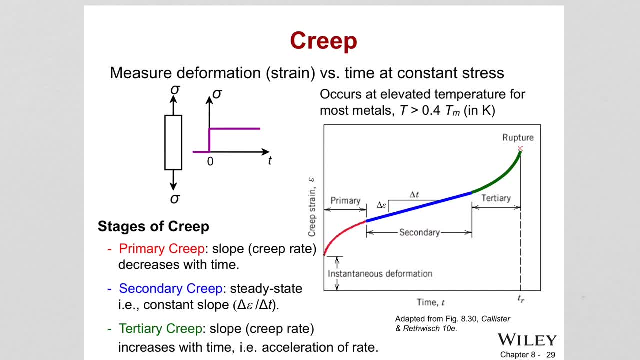 At some points. So what happens then? It fails, And so this was an example- to creep, And we said it usually happens at high temperatures. So where there is a high temperature application, such as in jet engines, generators, we need to be careful about the creep. 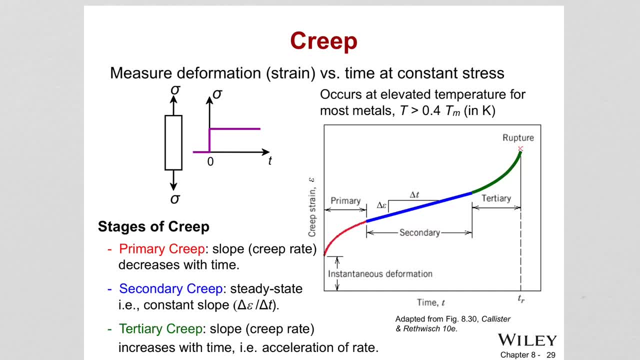 So again, even if you have a high temperature application, you need to be careful about the creep. Even if the stress levels are much smaller than the yield strength of the material, materials can still fail with creep, And the creep temperature is usually 0.4 times of its melting temperature. 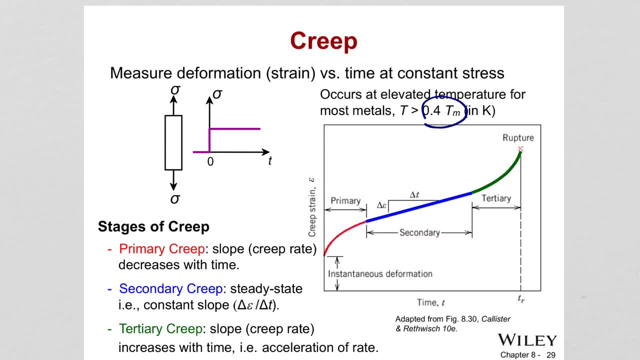 So if the melting temperature is 100 at 40 degrees, you need to be careful about the possible creep failure. So how do they measure the creep behavior of materials? So they look at the creep strain, basically the strain happening with time for a certain material. 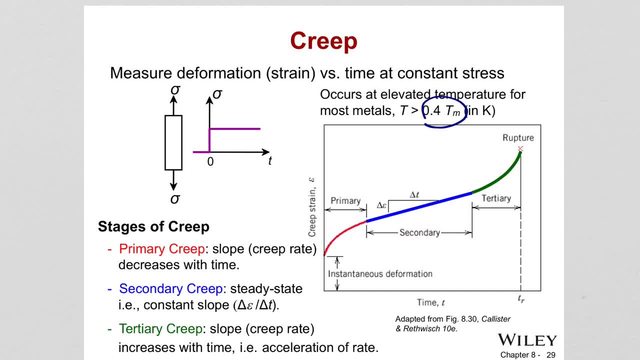 And then they record the group, they plot and record the data. And here we are seeing such experimental result And based on that we observe three stages of creep. So at time zero there is instantaneous deformation, which is the elastic deformation right. 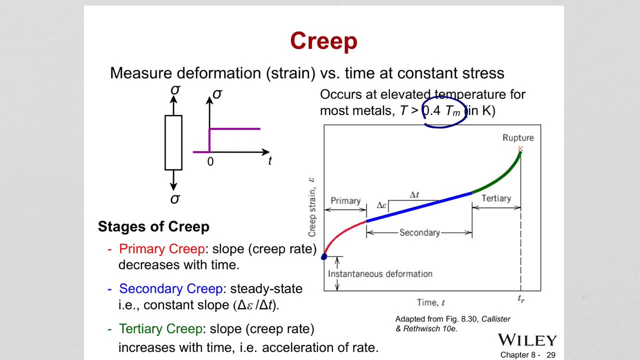 And then, with time, The plastic deformation will start. So creep is, remember, it's the plastic deformation happening with time. okay, So, and it will show a behavior as such, like this: So in the first region, which is the primary region, the slope is decreasing right. 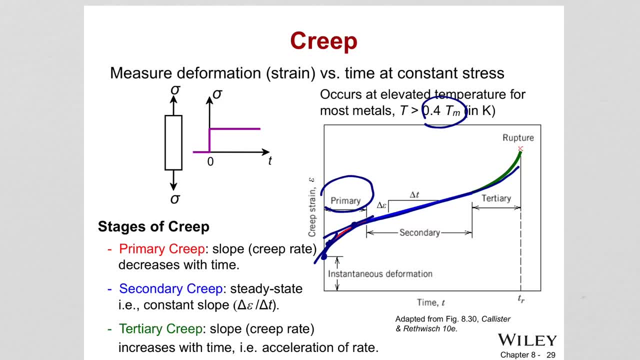 The slope is decreasing, So the creep rate is decreasing with time. Therefore, the creep rate decreasing with time, because creep rate is basically strain over time. right? This this over that is going to tell you what the creep rate is. All right? 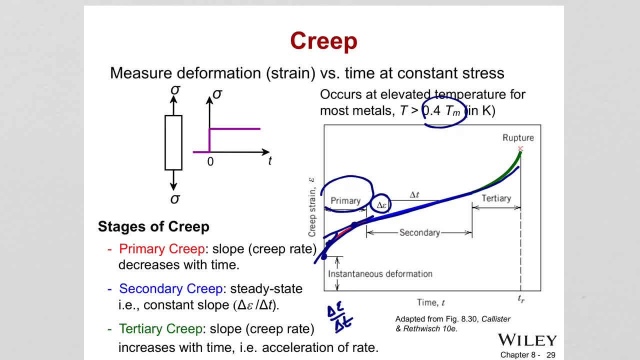 So why is it decreasing with time? In the first region, which is the primary region, the slope is decreasing with time. So remember, when the material starts to deform plastically, it will actually is going to expose to strain hardening. 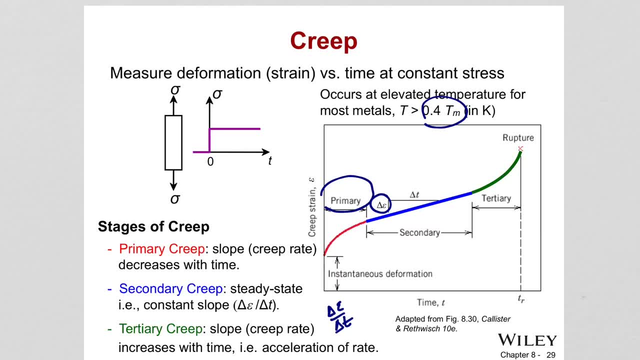 So it's going to get stronger. That's why, once the plastic deformation starts here, the creep behavior is going to be with a slowing down speed. So that means that because the material is getting stronger, That is the behavior we observe in the primary creep region. 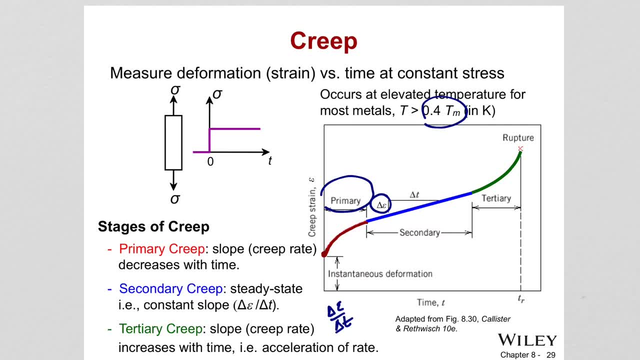 The most important region is secondary creep region, because that is where the material spends most time in. So what happens here? We observe a steady state creep behavior, meaning a linear change of the strain with time, And of course the slope is again delta epsilon over delta t, which is constant throughout this stage, as you can see. 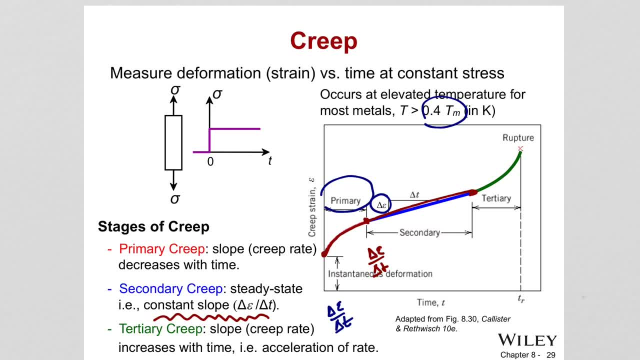 And the final stage is tertiary creep. the third stage, And of course this is where we go to the fracture Basically. at certain, At certain point, when the necking begins, the sudden failure happens in the fracture. So this is the third region, right?